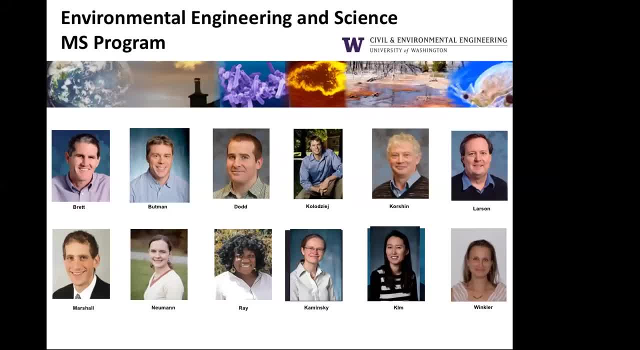 Okay, welcome everybody. We're about to get started here. I'm Eric Huberti. I'm one of the graduate advisors here. Thank you for joining us. As the information session goes on, you should see a little chat box in the bottom of your screen. 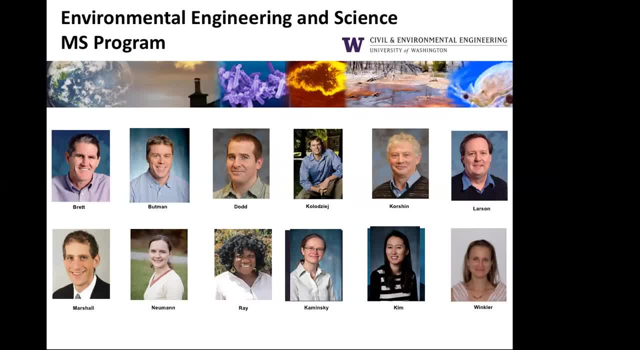 Feel free to put questions in there. If they're pertinent to what's being talked about at the time, I'll interject and ask those questions on your behalf, And then, at the end of the program, we'll have some time for a Q&A, And so feel free to throw questions in there for that as well. So, without further ado, I'll let Mike introduce himself. 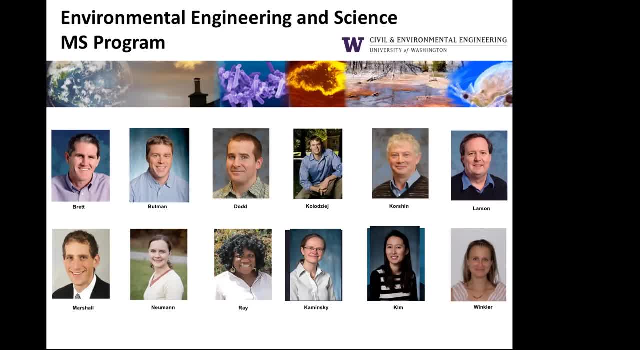 Hello, my name is Mike Brett. I'm one of the environmental faculty. I'm also a couple of different things, I guess. I'm the graduate program coordinator for the department And I'm the associate chair for educational issues in a department. 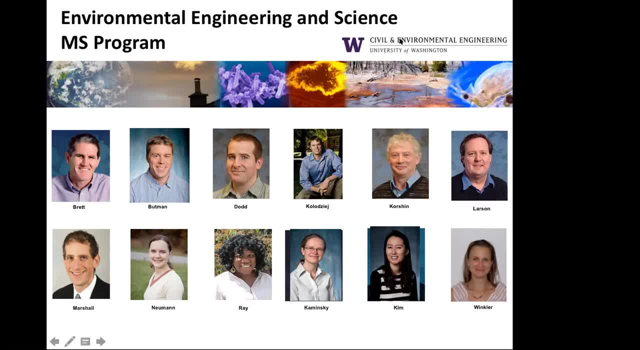 And I'm also one of the characters in this group of pictures here. So we have. let me count. we have 10 faculty in the environmental group. I'm the first. I'm the first one on the upper left-hand corner. I work with lakes and eutrophication lakes. We have David Buttman, who works with a carbon cycle. He has a joint appointment with the School of Environmental Science and Forestry. We have Mike Dodd. He works with oxidation reactions and drinking water systems. 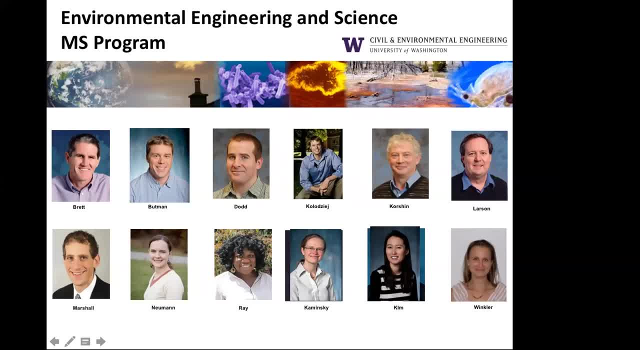 Ed Kolodziej, who works with pharmaceuticals and other anthropogenic contaminants, gagefablesedu and dams of the In surface waters and groundwaters. Greg voskkyim, who works with corrosion. Greg voskkyim, who works with corrosion. 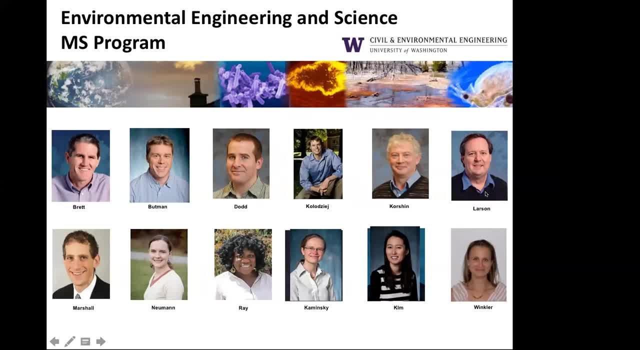 In water distribution systems. primarily Tim Larsen, who's an air pollution salient marshal, is salient marshal is an air pollution impacts sortof person. He studies the impacts of air pollution on different socioeconomic groups. Professor Rebecca Newman studies groundwater contamination, especially with. 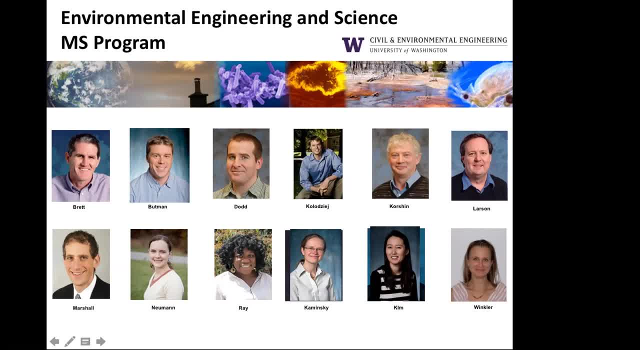 disgusting plants, etc. arsenic. Jessica Ray is our newest hire. Professor Jessica Ray just started in our department about a year ago and she works with stormwater and contamination of stormwater. Professor Kaminsky has been here for a few years. She studies drinking, not she studies. 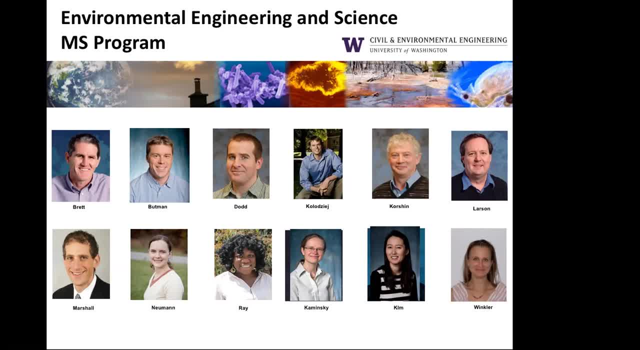 sanitation in developing countries, so especially sanitation in like refugee camps and places like that. How do you deliver that in an effective way? And Amy Kim does research on low-impact development and Professor Mari Winkler does research on the nitrogen cycle and it's particularly 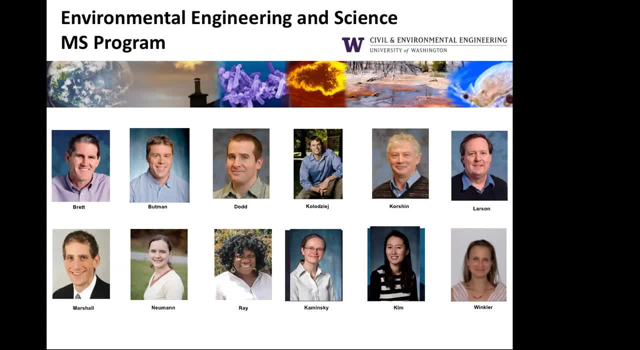 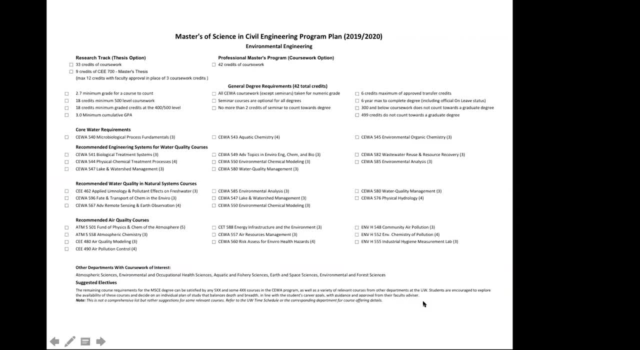 in water treatment systems and nitrogen removal and anammox. I'm going to change my slide, Sorry, we had operator air there for a second, So right here is a program plan for the professional master's program that we offer within the environmental group, and it outlines: 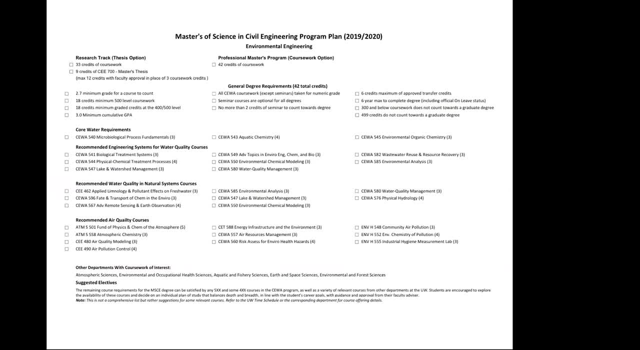 a couple different tracks you might want to take and it specifies the overall requirements. We're on a quarter system at the University of Washington, so it requires 42 credits of coursework and there's a if. it's just, not just, but if it's a coursework based only, it's 42 credits, of course. 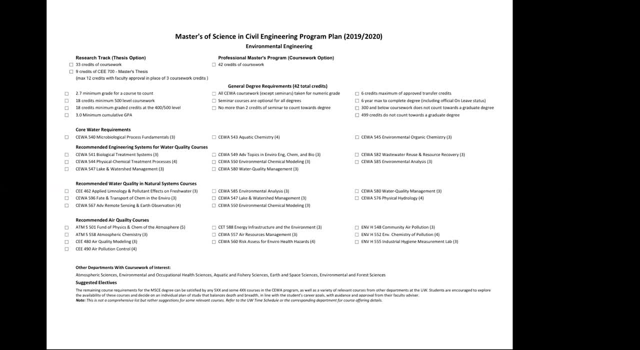 if you end up doing a master's research project as well, then it's 32 credits of coursework, nine credits that you get from your thesis. There's some requirements you need to get you know: half your classes have to come from or 18 credits have to come from. 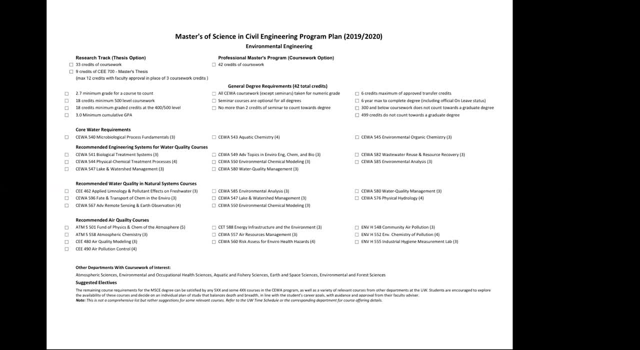 graduate-level classes. The rest can come from senior and graduate-level classes. You have to maintain a minimum GPA, overall GPA, of 3.0.. You have to get at least a 2.7 in every class and we have um three required classes for the two water tracks. We have two basic water tracks. One is 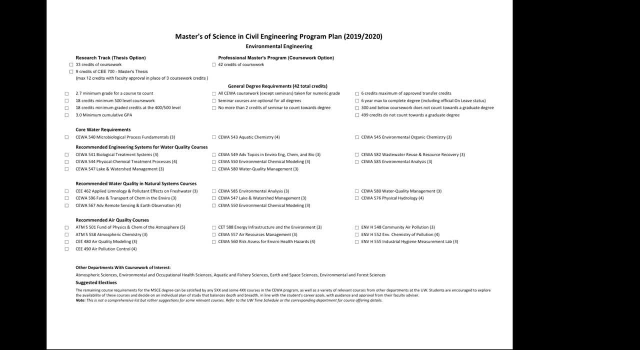 water and engineered systems and the other is water in natural systems. I'm more of kind of a natural system person. We have a lot of people interested in stuff like streaming restoration but you know probably two-thirds of the people in our program are coming from are interested in. 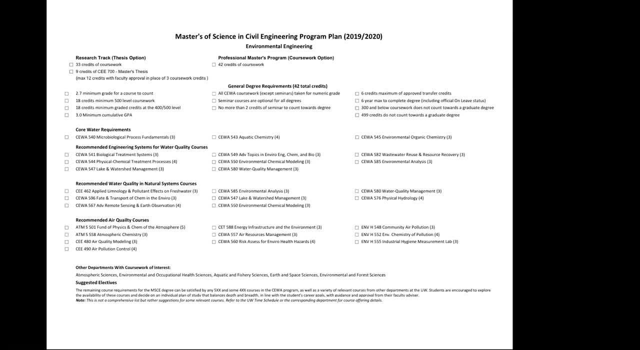 going into some type of engineered water treatment system like drinking water treatment, wastewater treatment, stormwater treatment, something of that sort. One thing about our program that I think is fairly unique and is a little bit different from other master's programs in this department. 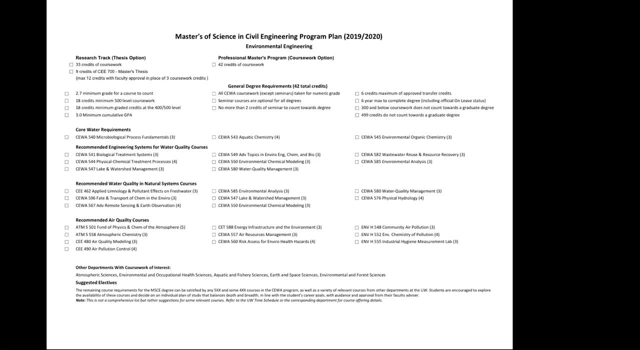 is that we do attract students from many different backgrounds. So we have a lot of students that come from non-engineering backgrounds: geology, you know, chemistry, environmental science, what other? oh, we've got lots of different departments that contribute students to our, to our, to our program. So we have- it's- a very diverse group of graduate students and and and, and especially in the environmental group. 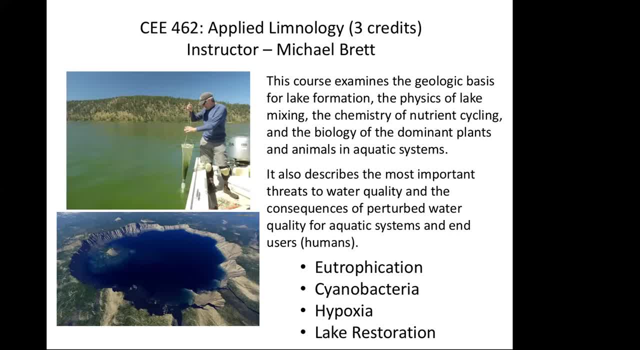 Um. so some of the classes that we offer for for people um one is the class I teach um applied limnology and that class focuses on on eutrophication. the most common um disturbance of um of surface waters, of inland surface waters, and there's a picture of 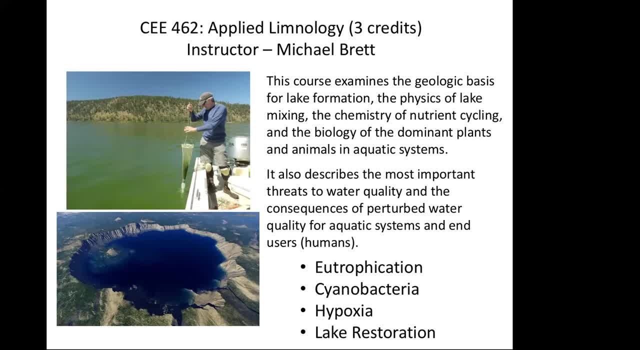 me collecting a sample from uh Upper Klamath Lake in Southern Oregon, uh, which has some of the worst blooms in North America and is only about 25 miles away from um Crater Lake, which has the highest water quality in North America. 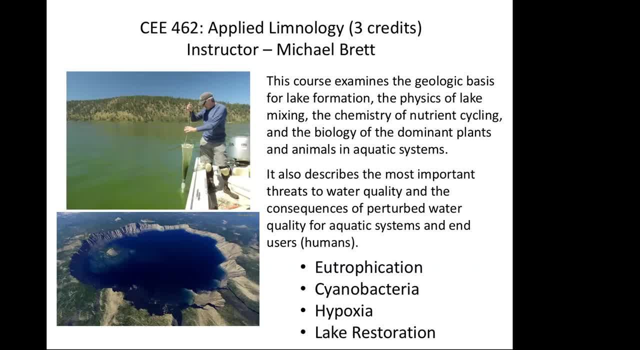 So we have two lakes that that have the almost completely divergent water quality, located about uh 25 miles apart, and one is connected to the other. uh Crater Lake discharges to Klamath. Um, then we have uh. one of our required classes is microbial. 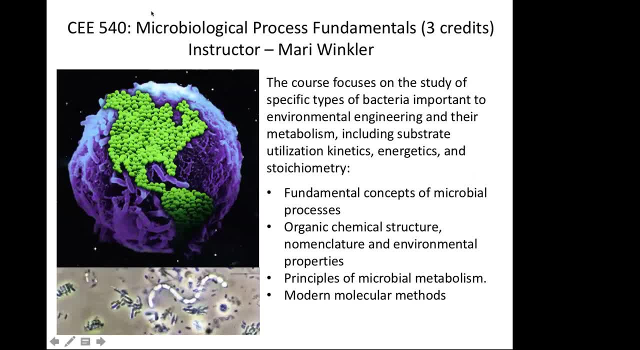 um process fundamentals taught by Professor Mari Winkler, and um this gives you, uh, a very strong foundation on on what bugs do in engineered systems. A lot of of the water treatment done in engineered systems is done by bacteria. 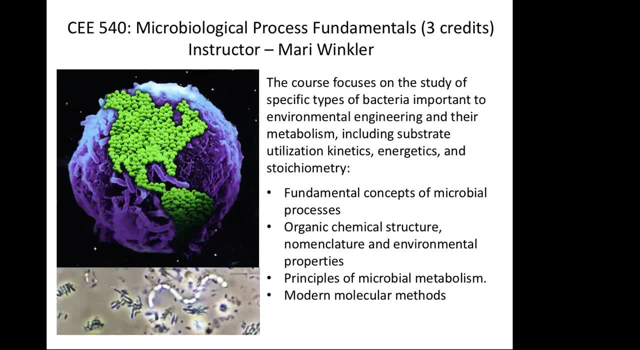 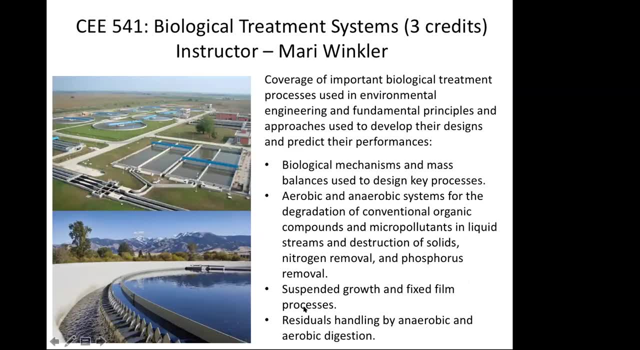 and this class will teach you what you need to know about bacteria so that you can be an effective environmental engineer. Um, um, we also have a class on biological treatment systems. it's got Mari Winkler listed as the instructor, but the last two years we've actually had a professional engineer teach it, which I think is really good. 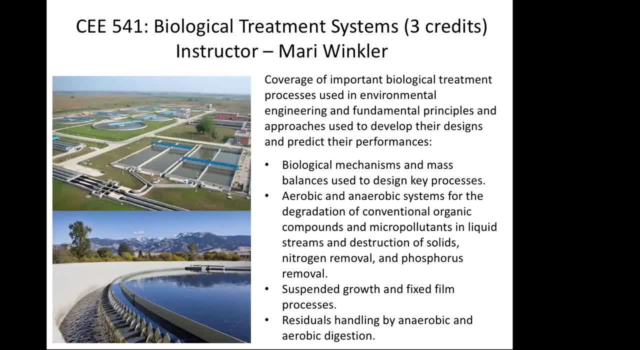 They bring the practical perspective of actually designing water treatment plants- drinking water, I mean, wastewater treatment plants- um to this class and uh I think it's uh very useful for the students to see kind of the first-hand perspective of how a professional engineer would um approach these sorts of problems. 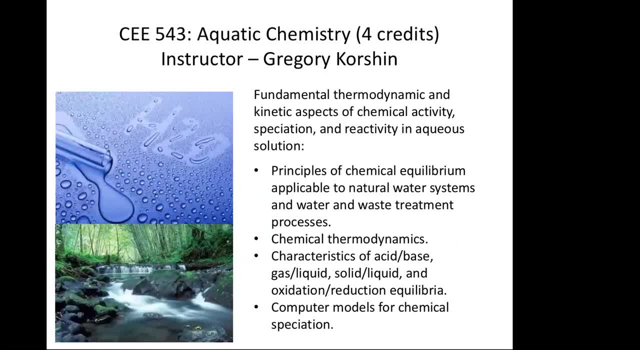 Um, aquatic chemistry is another one of our core required classes. that's taught by Gregory Corsion, so that's going to give you a very strong foundation in environmental chemistry. Um I, this right here is probably the key core class in our curriculum. 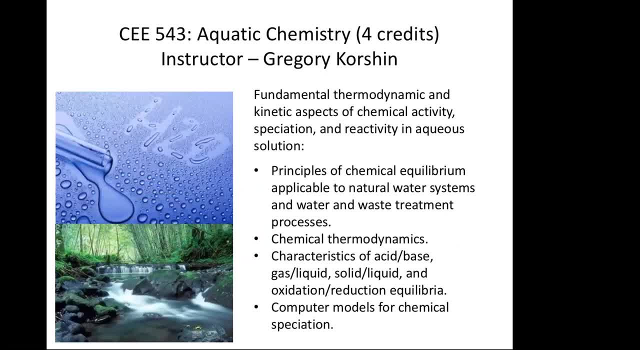 Most students say they during the quarter when they take this class, they spend as much time on this four-credit class as they do um their other. you know classes put together so it would take, you know, four credits of this and eight credits of other stuff, and 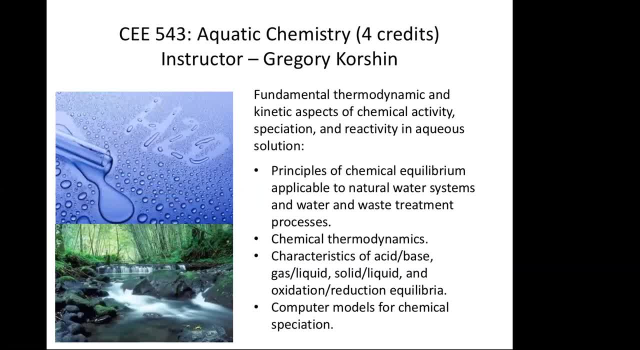 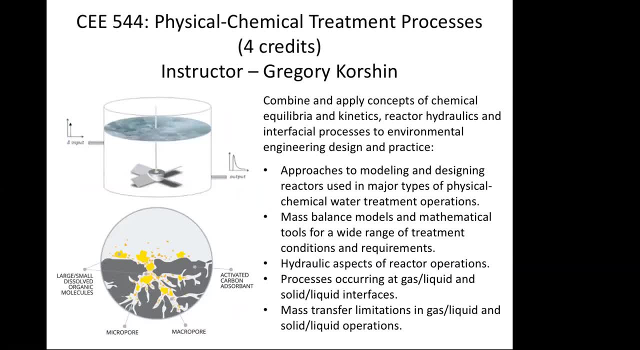 this class is probably more than half the work that goes into that quarter, but it's a very important foundational course for us. Um physical chemical treatment processes, also very important for understanding um, especially um drinking water systems. Um. 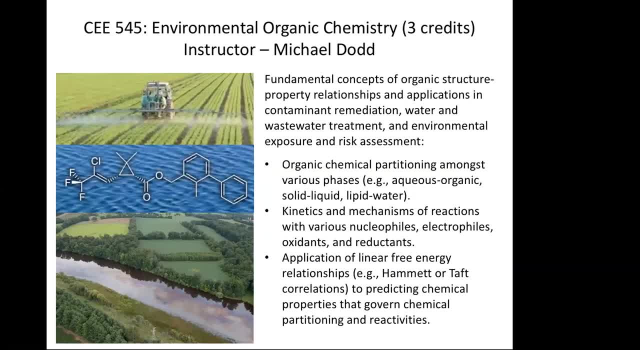 so that's also taught by Professor Corsion. Um, environmental organic chemistry is taught by Mike Dodd. Um, he's, uh, like I say, one of our. he's our, our, um, our big, um organic chemist person in this department. 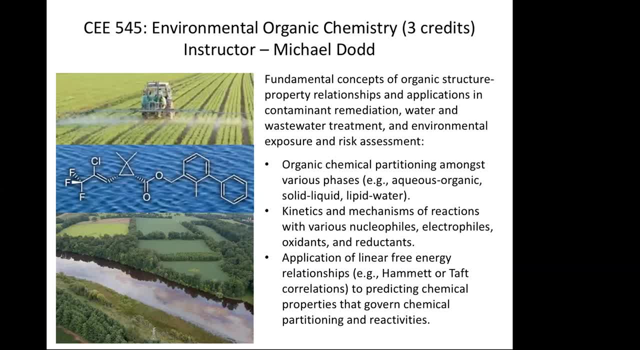 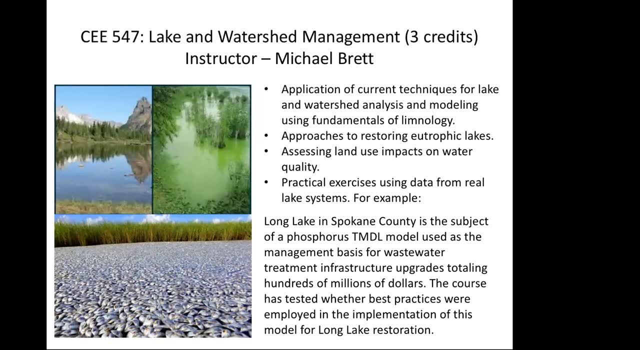 This is also one of our our core required classes. so our, our four, our three core classes are microbial process fundamentals, aquatic chemistry and environmental organic chemistry. And then um graduate class is taught by me, called uh Lake and Watershed Management, and really what this class is. 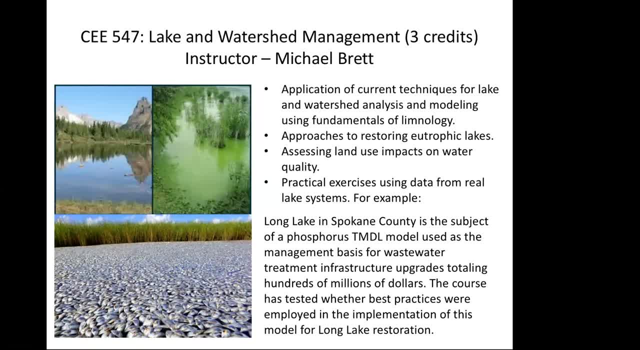 is it's uh best professional practices for environmental modeling. so we teach students how to um, assess and vet in uh environmental models to figure out whether the environmental model is properly characterizing the system it's being used to represent. 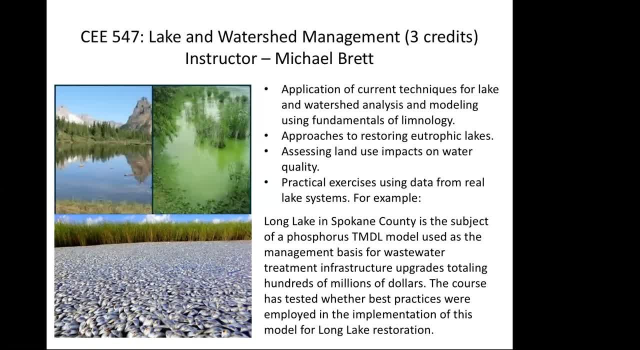 So people oftentimes just pull models out of boxes and, just you know, start using them, And this class will help you develop the tools so that you would know whether a model is actually, um, a fairly robust representation of the system it's being used to manage, or 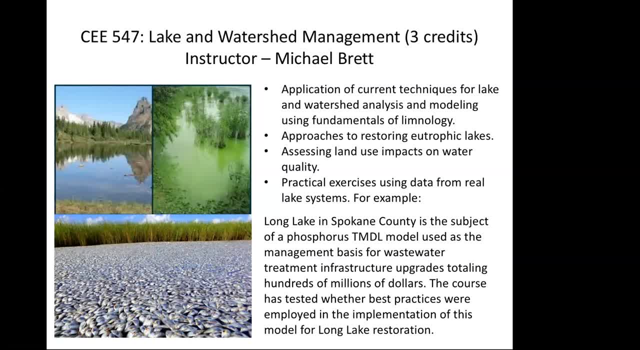 or if it's not. it's important to know that because if you're going to spend a lot of money um managing a system on the basis of environmental models, you want to be fairly confident that the environmental model is is is a. 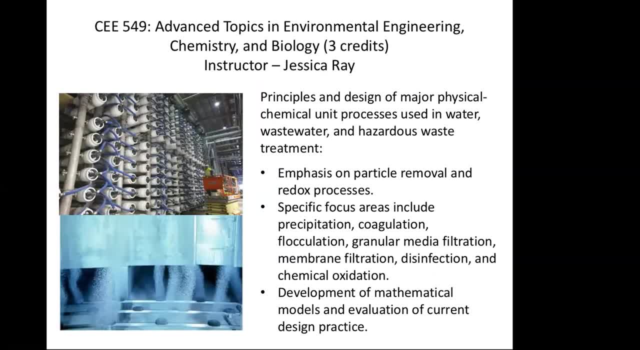 is a fairly good representation of the system that you're interested in Um advanced topics. So that's uh going to be taught by our newest professor, uh, Jessica Ray, And I think, at least initially, she'll probably be covering a lot of topics that are related to. 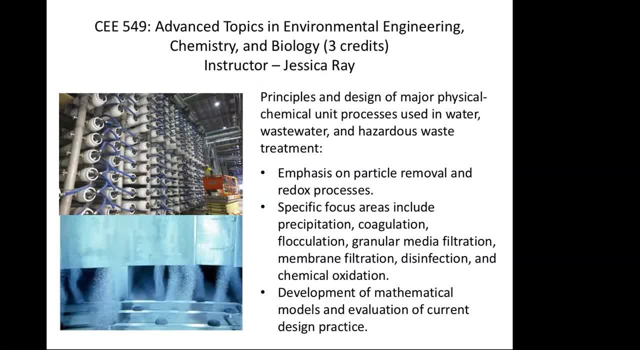 um some of the more innovative techniques that are coming out there for stormwater management. There's a lot of interesting uh ideas on on how to deal with stormwater There's in the Seattle area there's a huge amount of money being spent on issues related to stormwater. 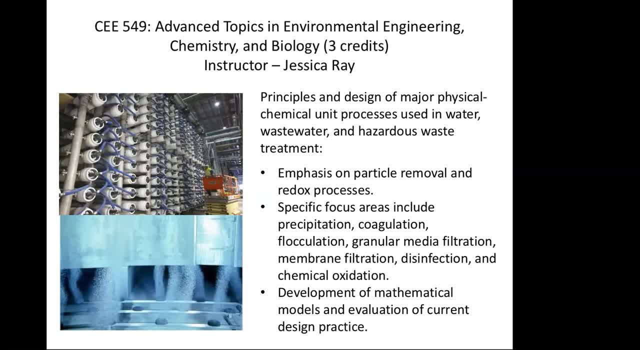 There's um a huge push by both um King County Metro and uh the Seattle Public Utility, Seattle SPU, to um deal with combined sewer overflows, And so both Seattle City and King County are spending about $1.5 billion dealing with CSOs in the next decade. 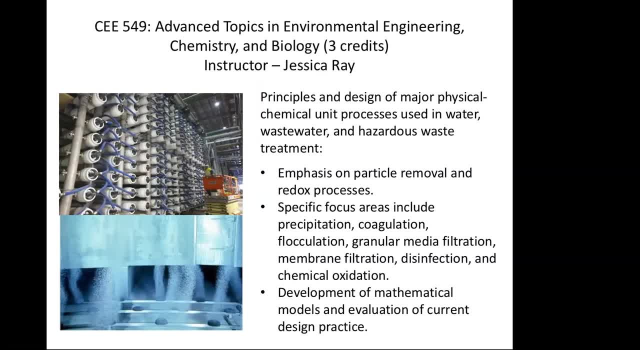 So there's a whole lot of uh infrastructure being put in place. There's a lot of research needed to to support that infrastructure And there's a lot of really interesting challenges associated with the. the quality of water- Um, you know, the low quality of stormwater and the low quality of of of these CSO discharges. 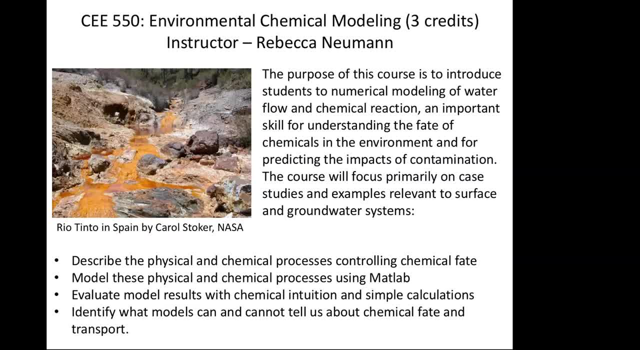 Um. another class is environmental chemical modeling by Professor um Rebecca Newman, And I mentioned her earlier. She uh does a lot of research on um the mobilization of arsenic in groundwater systems and in different parts of the world. 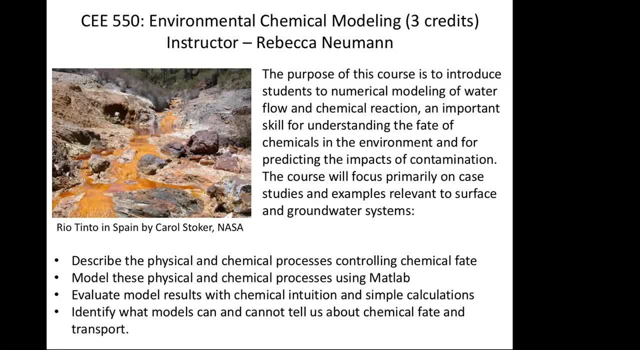 But a lot of her work has been done. Uh, in Bangladesh, where they have real major problems with arsenic contamination of groundwater systems, And so a lot of that is got to do with um, redox conditions and how those affect the solubility of of different constituents in groundwater. 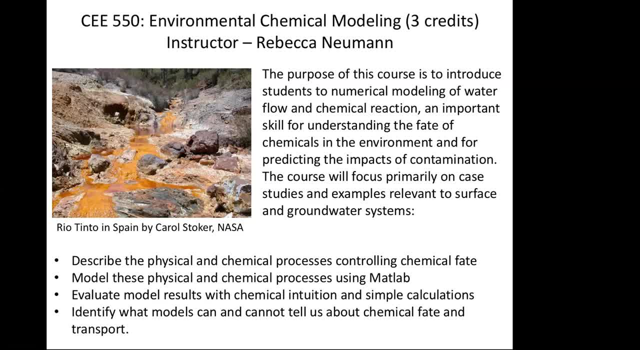 So arsenic is much more soluble, uh, in anoxic conditions And and and. so Professor Newman helps you understand how to represent that, and, you know, using mechanistic models, numeric models. Um, that's the end of what I have. 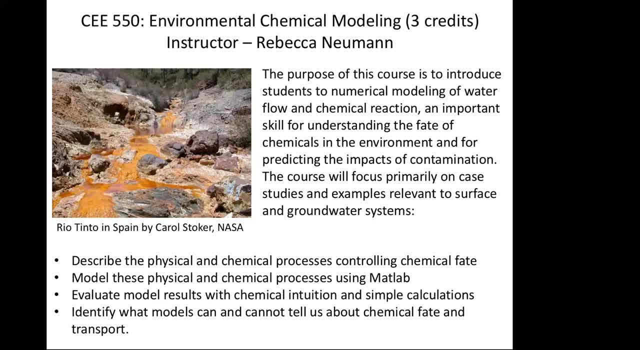 To say right now. I want to say a few general things about our graduate program that I think are worth knowing. One of the things that we're trying to do with our graduate program that I think will help out um incoming graduate students is that we're trying to line up the coursework that we offer in our in our program. 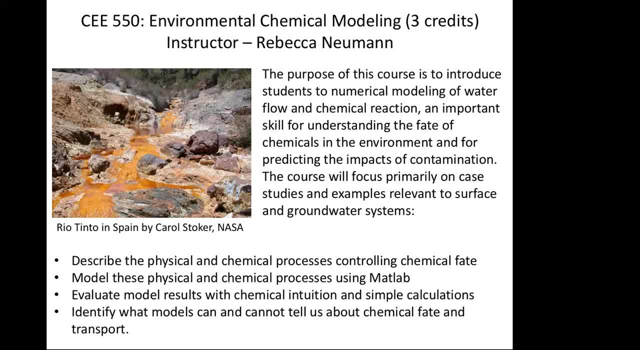 So that um um graduate students can take all their classes either on Monday or Wednesday or, alternatively, take them all on Tuesday and Thursday. So In some quarters we'll we'll strive to offer all our classes on Monday and Wednesday, and other quarters will strive to offer all our classes on Tuesday and Thursday. 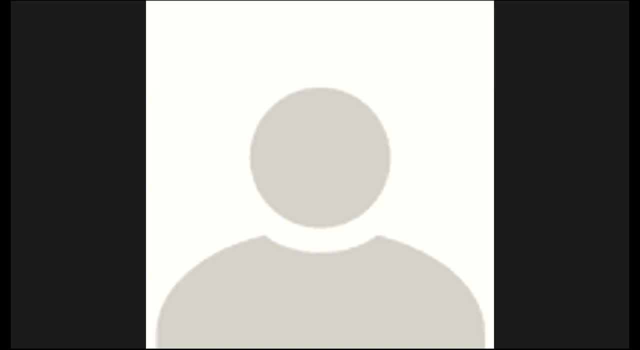 But within a particular quarter. there we're going to try to offer all the classes on the same two days, And the reason that we're trying to do that is because a lot of the students that enter our professional master's program are working part-time in some of the local engineering firms. 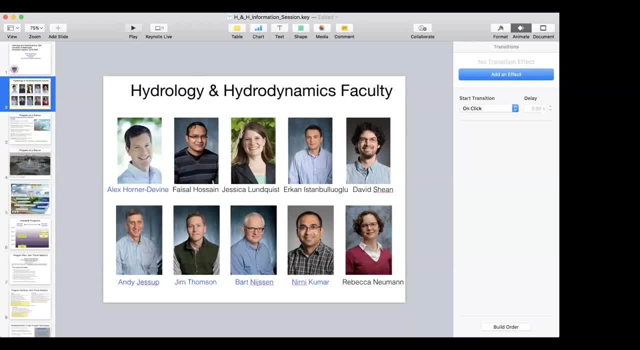 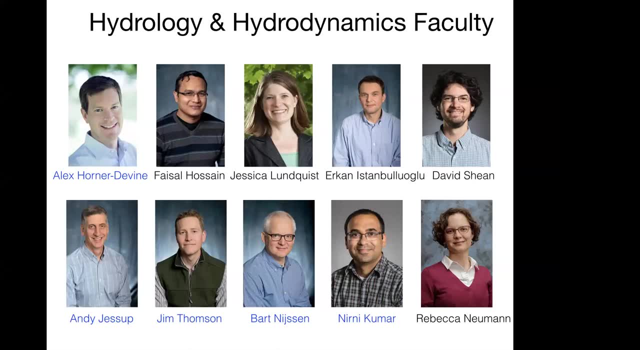 The job market in Seattle right now for environmental engineers is is actually fantastic. I don't know else How else to characterize it. Everybody's getting jobs and a lot of people get part-time jobs that they do while they're while they're in graduate school. 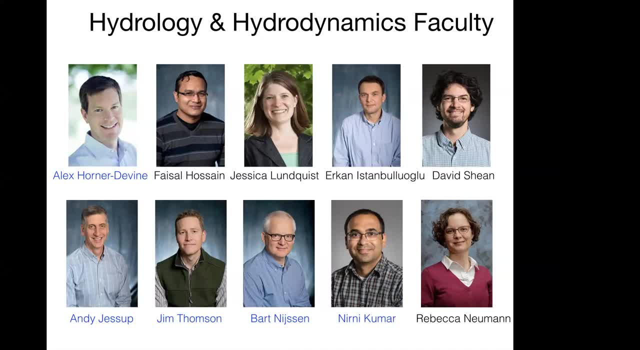 They develop- you know, some, you know- rapport with the local firms- uh, get to know what's going on around here, And they want to be able to have their work week set up in such a way where they can focus some days on their- you know- part-time job and other days on their courses. 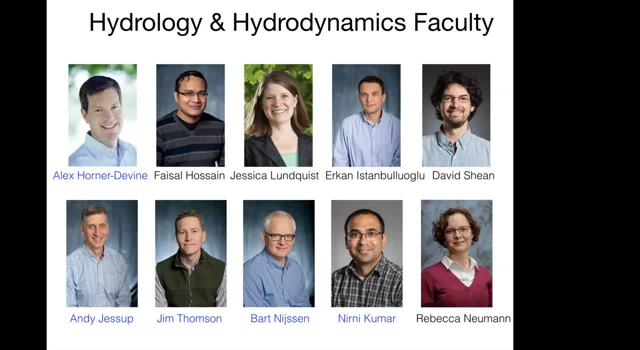 And so we're working really hard to try to to make to accommodate that, And I think we're making some good progress. We're pretty close, Close to that. The other thing that we've done recently to help out graduate students in the department is that we've turned over our entire seminar series to be operated and run by the graduate students. 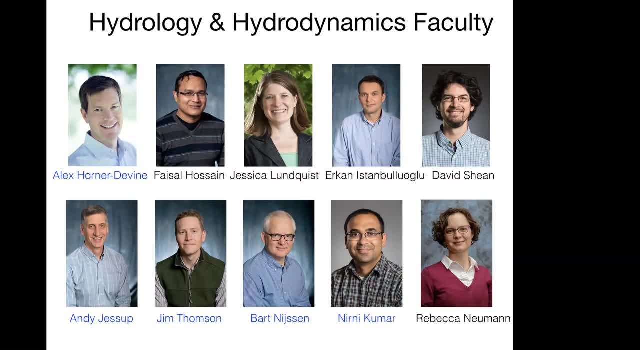 And we've had a tremendous boost in the interest in the graduate seminar series. Now that we've turned it over to the graduate students, they apparently are capable of picking much more interesting seminar speakers than professors are, And so we're trying to do some things to really improve the experience for students, for 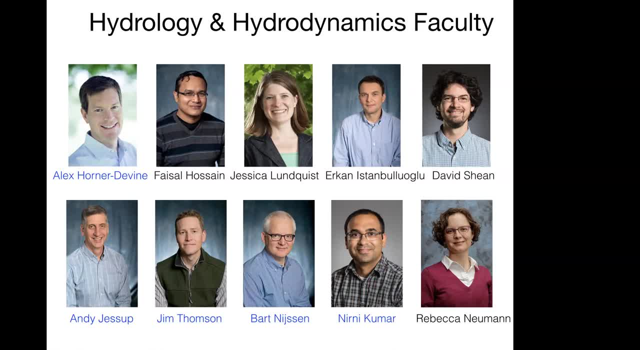 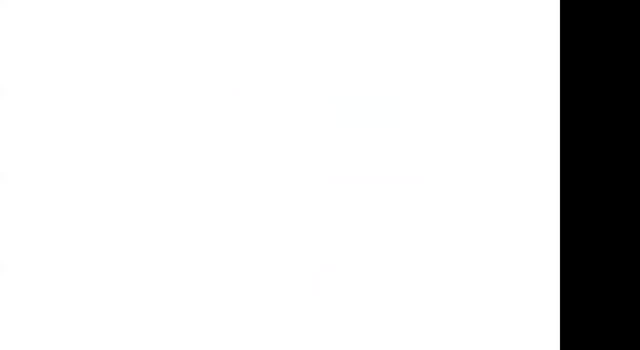 For graduate students in this department. So that's what I have to say for now. Now Professor Erkan Istanbuli is going to speak about the hydrology and hydrodynamics group. I'm not muted, right, Am I okay? Good, 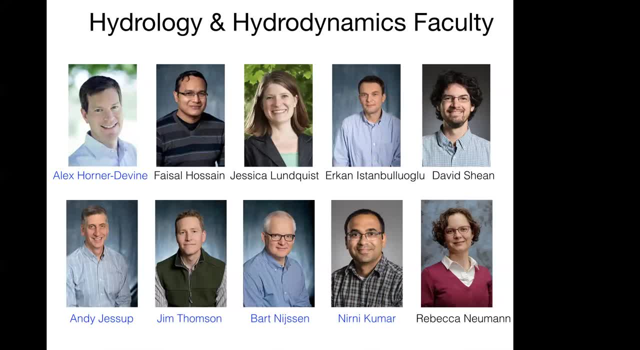 Okay, Hello, My name is Erkan Istanbuli. I'm a professor in this department. I'm in the hydrology and hydrodynamics area, So this is essentially that we have five, ten faculty in the hydrology and hydrodynamics area. 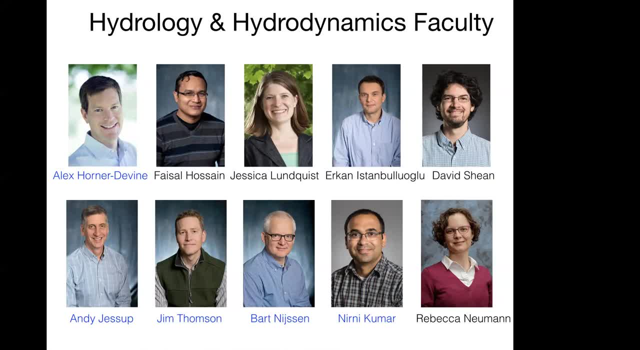 Alex Horner, Devon, is in hydrodynamics and he works on. he studies plumes in rivers and estuaries. Faisal Hussain, he's a hydrologist and he focuses on satellite remote sensing water management projects In developing countries. Professor Langquist works on primarily works on snow and atmospheric. 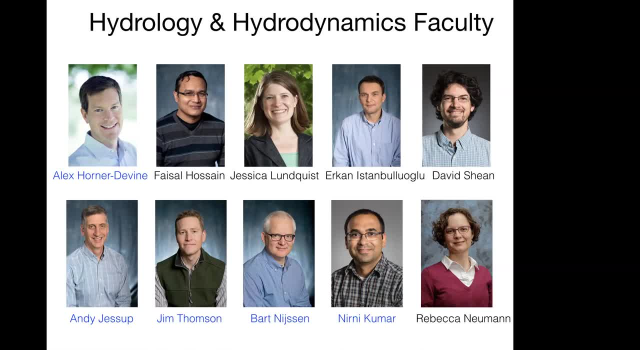 modeling as related to snow and extreme events, And I am I'm a hydrologist and I work on mostly hydrological modeling: ecosystems modeling and modeling of geomorphic processes in relation to snow, Geomorphic processes, Geomorphic processes in relation to hydrology and ecosystems. 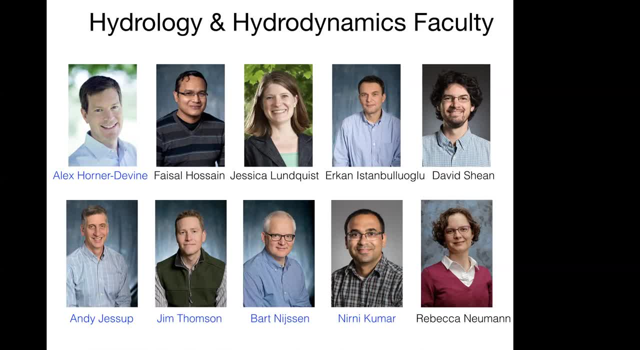 And I have a growing interest in the built environment as well in the context of net zero, carbon neutral concepts. And David Sheen is Professor Sheen. He is one of our newest members. His area is on satellite remote sensing and remote sensing through unmanned vehicles like drones and other things. 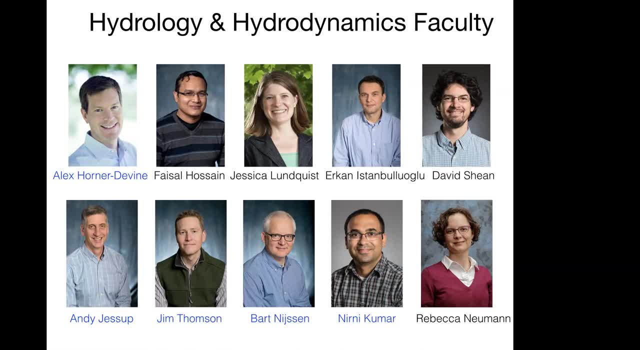 I mean he has a great tour shop. that I mean he flies drones and he collects a lot of data at less than a centimeter scale resolution And he analyzes the data sets with respect to changes on the landscape and so on. And Professor Jessup is in the Hydro. 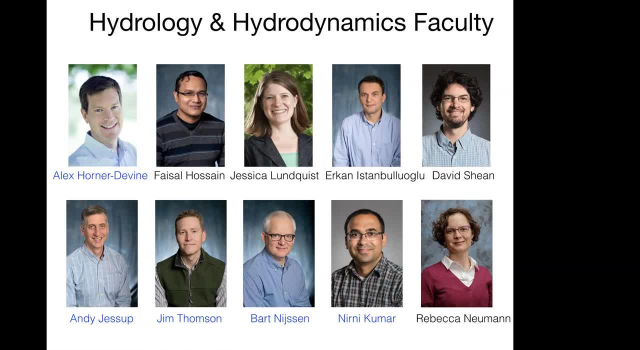 Dynamics group. He focuses on oceans. Professor Thompson also in the Hydro Dynamics area and he is largely interested in harnessing energy from waves. Professor Knysen runs the computational hydrology group. He has a fairly large modeling group. He is largely interested on climate change impacts. 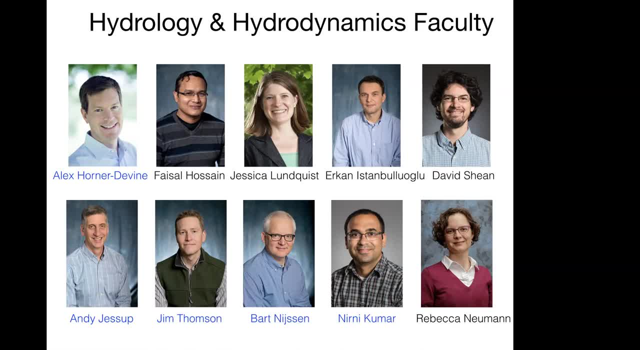 on hydrology and water resources. Thank you. Professor Kumar is interested in hydrodynamics modeling, setting up very sophisticated models to examine flow dynamics and sediment transport and rivers and oceans in coastal systems. Professor Newman is sort of the joint member between our Hydrology and Hydrodynamics group. 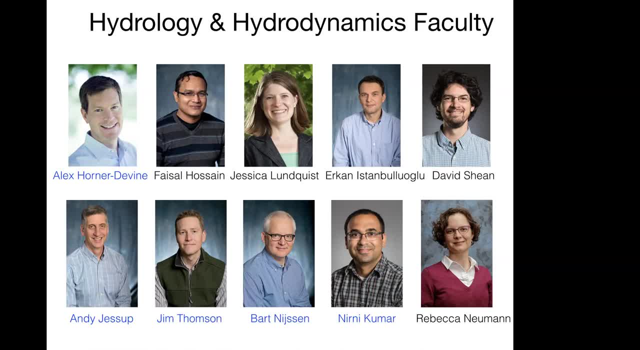 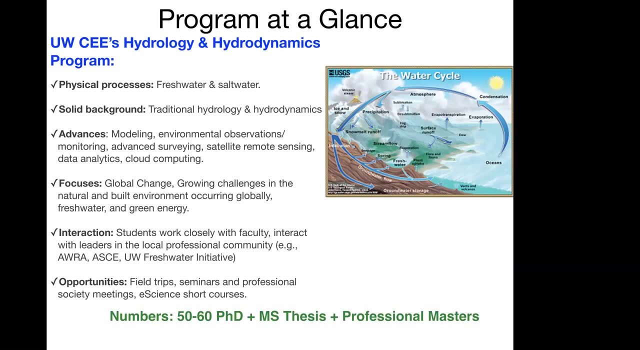 and the Environmental Sciences group And she studies groundwater and groundwater contamination with respect to arsenic And she has a lot of interest. And she has a lot of interest in the global developing world. Our program- sort of a summary of our program. 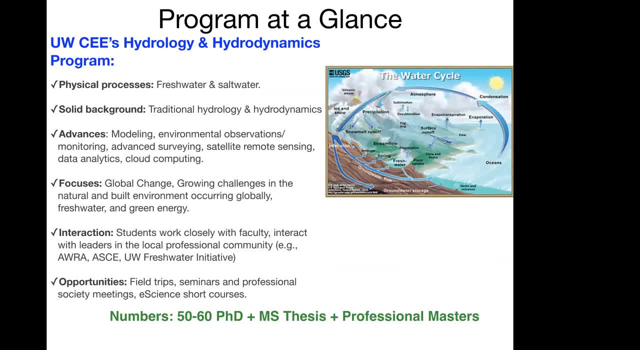 is that in our classes we focus very fundamentally on physical processes. You would have a very sound physical understanding of the freshwater and saltwater in general within the context of the landscape and in different reservoirs of the landscape, Building on this sort of traditional hydrologic hydrodynamics. 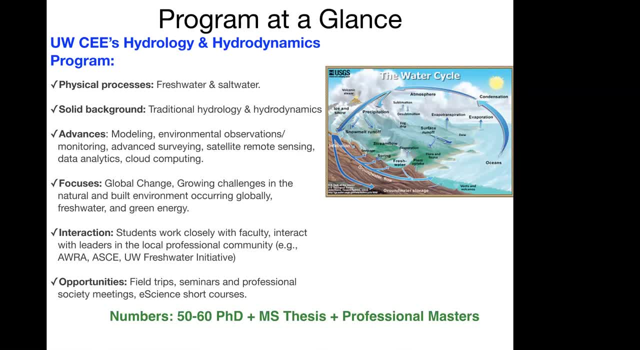 understanding. we also use more advanced methods like modeling, environmental observations and monitoring in combination with modeling, advanced surveying, satellite remote sensing, data analytics and cloud computing. in our classes, You will see that some of these classes would be focusing on, let's say, satellite remote sensing. 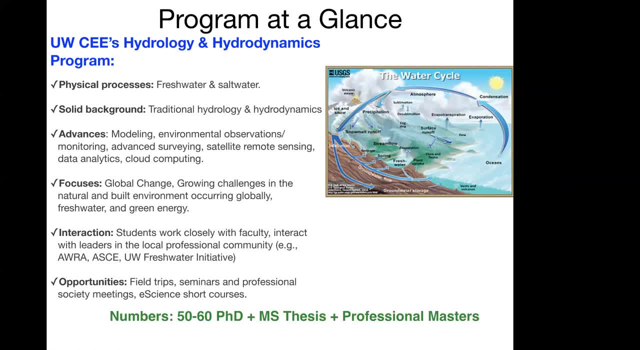 and surveying. But some other classes would be using that satellite remote sense data for calculation of certain hydrological or hydrodynamic phenomena. And more and more we start integrating data analytics, In other words sort of the big data science and computation in our classes. 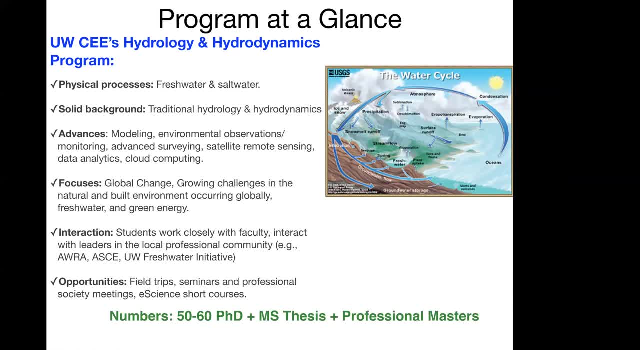 We broadly focus on global change questions like growing challenges in the natural and built environments that occur globally within the increase of population and climate change. We study freshwater resources across the globe And we're also interested in energy from water and waves and sort of within the context of green energy. 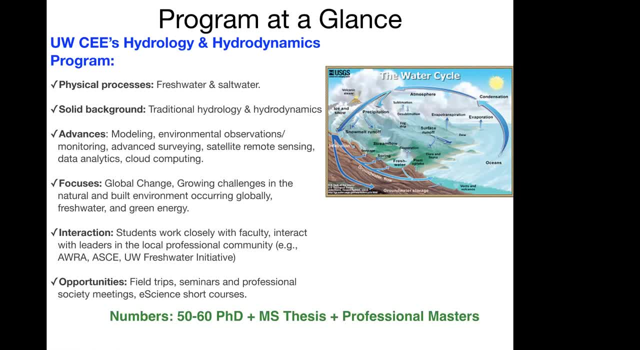 With building on these solid background and modeling and technology expertise. you would also have a lot of interactions within student groups. student-to-year work closely with faculty. We have one-on-one meetings with our students, whether you have a PhD student or a master's student. 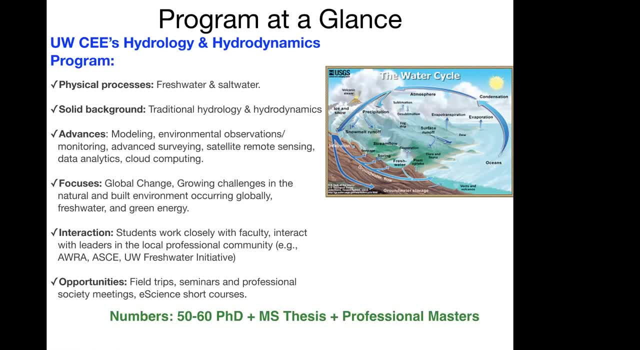 We always interact with you on a weekly basis essentially, And we also have local professional committees such as the American Water Resources Association and American Society of Civil Engineers, student chapters that focus on hydrology and hydrodynamics field, And we also have 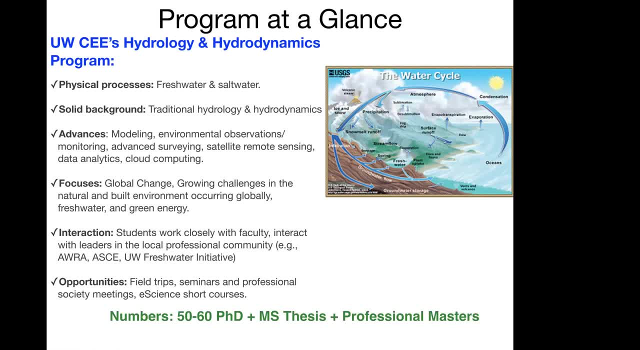 OK, And we have the University of Washington Freshwater Initiative. that is largely run by graduate students and professional master's students And they have their own meetings, They invite speakers, They organize seminars. It's a very interactive group and live group. So we have a lot of interactions to that end. 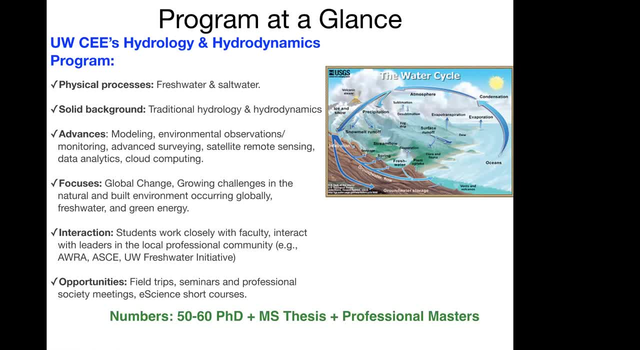 There is a lot of opportunities. We have field trips. A number of our faculty does field work and they may require help with the field data collection and analysis, And there's also opportunities in terms of taking short courses from e-science. Some of our grants involve developing short courses on modeling, big data, sort of data analysis and so on. 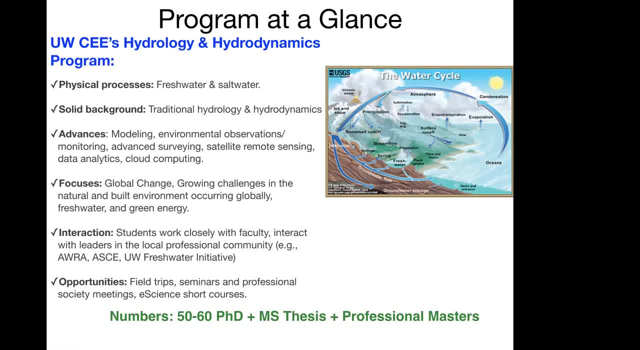 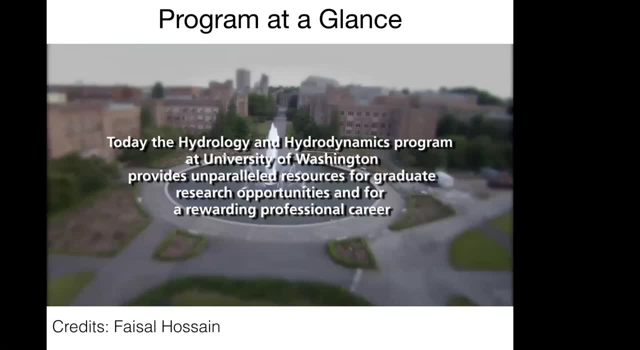 We work with e-science through those short courses. They are not listed in this presentation, but there's plenty of opportunities there through the Freshwater Initiative. This is a video that was developed by one of our professors, Faisal Hussein. I'm not going over this, but you can play it, so it sort of summarizes our group and our classes. 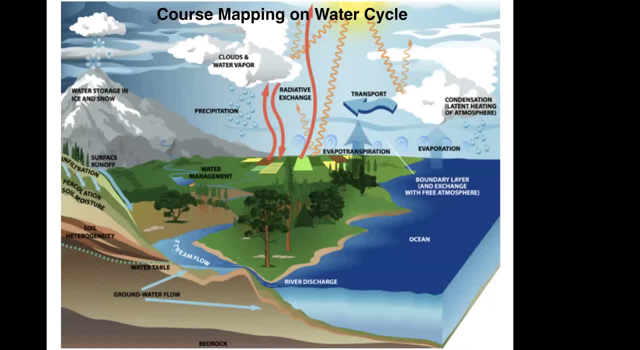 So I'm trying to map our courses on this hydrological cycle. We have the physical hydrology and snow. hydrology essentially looks at the from all directions We take the water all the way from precipitation in the form of rainfall and snow. We look at snow melt, how the water infiltrates into the landscape. 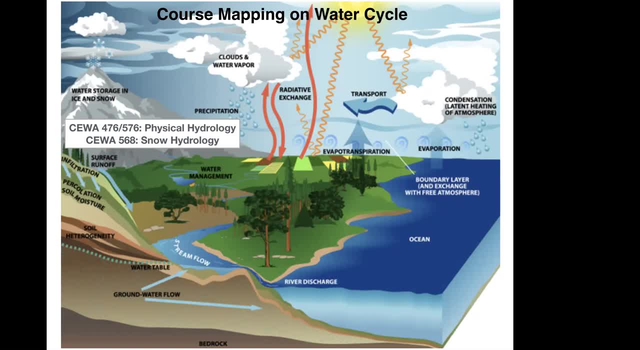 surface runoff processes, ground water runoff processes and so on. We take the water all the way from the mountaintops to the oceans. in these two classes, There's the data analysis course that intensely uses environmental observations with respect to water fluxes and other things. 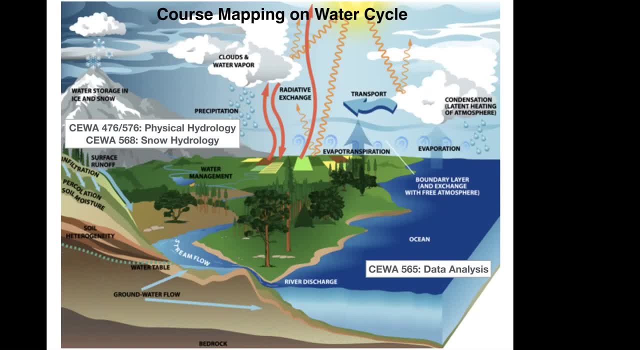 And it develops the basic concept of statistical analysis of water sources data and environmental data and builds on coding. Essentially they're using Python. in this class There's the ground water class that looks like the fundamental ground waters. We teach hydraulics of sediment transport. 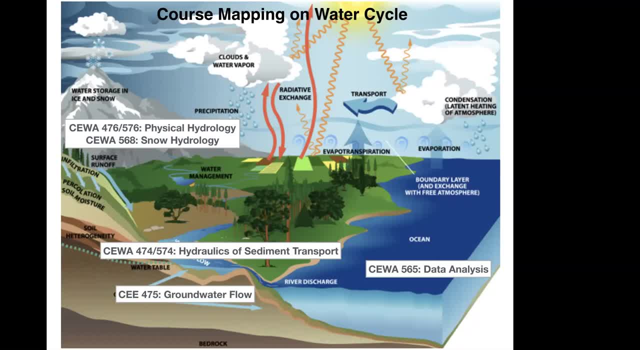 So when the water gets into the rivers, then this class takes the water from the tips of the channel, It takes the channel network from the groundwater and essentially studies how the sediment is transported within the channel networks And what is the role of, for example, rising limo of the hydrograph versus the recession limo of the hydrograph in the sediment transport and depositional processes. 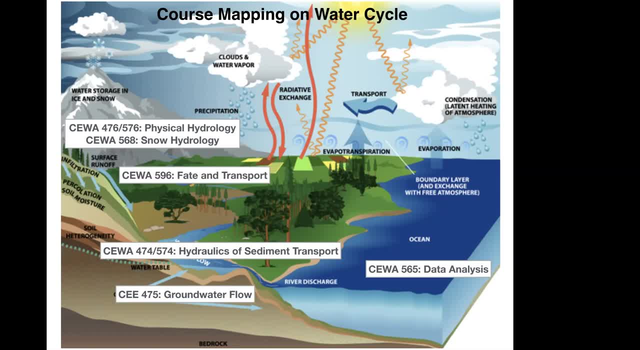 We have fade and transport. that was taught by Professor Neumann And this class looks at the conservative or non-conservative pollutants, How pollutants and sediment moves in the systems. in fluvial systems There's water management course that focuses on the water management projects. 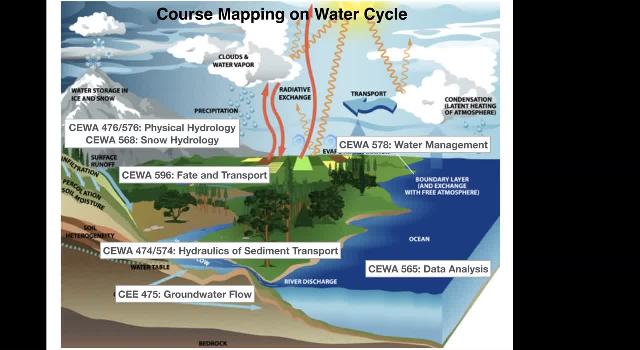 Managing reservoirs for residential uses, industrial uses And sort of gets into the concepts of programming like linear programming, dynamic programming, concepts In managing water resources seasonally and in terms of reservoir storage capacity. Coastal engineering looks at a lot of modeling in the coastal engineering class. 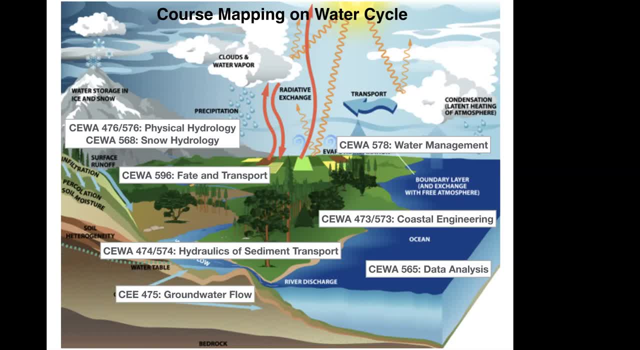 That looks at how the coasts respond to the forcing from the ocean through waves. Hydraulic design course is more specific to application of hydraulic design in urban environments In terms of collecting water for use, Wastewater and sewer systems and stormwater design. 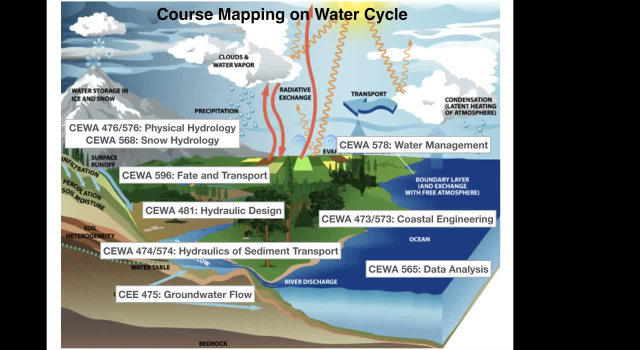 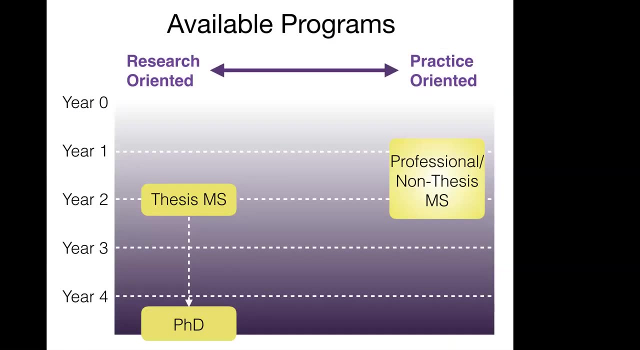 Green stormwater infrastructure and so on. There's an advanced hydrology course that looks at the more advanced topics In terms of modeling and statistical, in terms of process based modeling and statistical modeling- Our program, if you're interested in the piece. 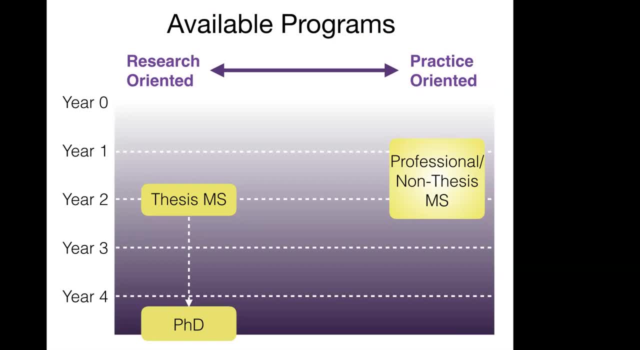 It's a professional non-thesis option. It is largely oriented towards essentially solving problems in the area of hydrology and hydrodynamics, So it's practice oriented. A number of our classes have examples that are directly related to application. While we have their fundamental theory, we have very sort of basic applications towards practice as well. 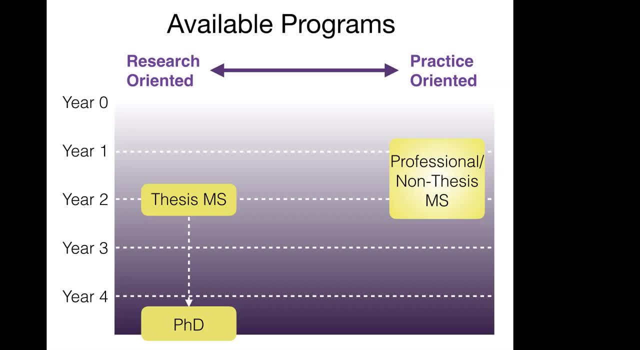 And you can complete this within. You can do it within a year, or maximum in two years, depending on your schedule, Because some people may want to work part time and take classes in two years. So it would fit on your schedule If you're interested in a thesis, master's thesis track. 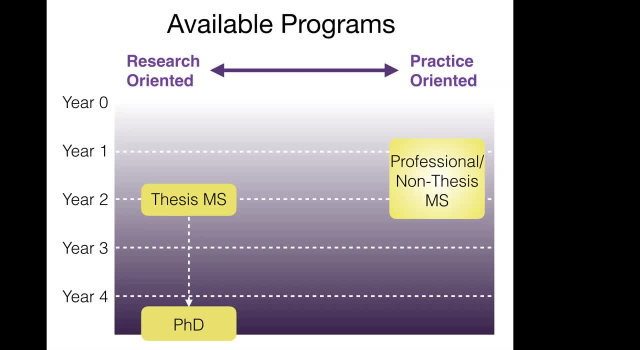 Usually it takes between two years, two and three years, Depending on whether you need to do a lab experiment or not and have your results go, But usually two years and two and a half years. Two and a half years is sufficient for a master's thesis. 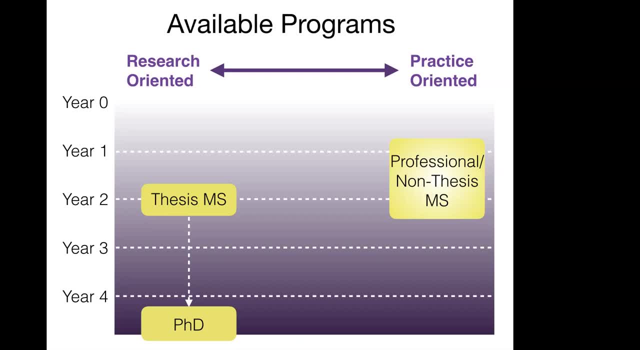 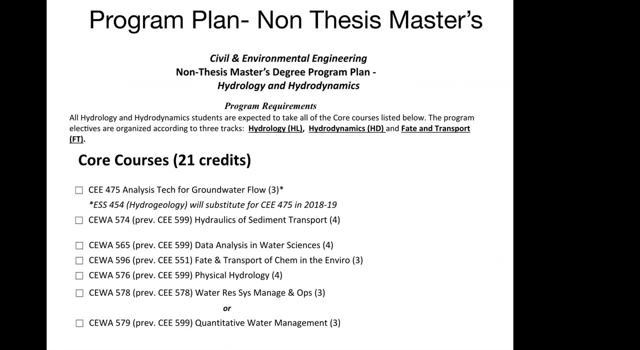 A PhD could take four years or five years, And it would depend on the research project. Like I'm not going to get into the details of the number of credits because Professor Brett already went over it, I don't want to go over time. 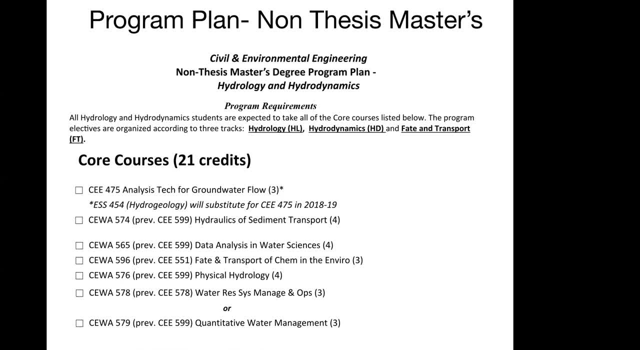 But we in our program and we have three main areas within the hydrology of tracks, Three tracks within the hydrology, Hydrology and hydrodynamics, And that are hydrology, hydrodynamics and fate and transport. You have core courses that we expect you to take for each of these. 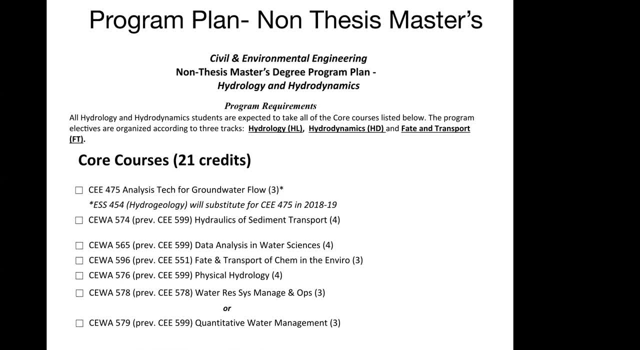 And there are 20 credit core courses that, whether you're doing hydrology, hydrodynamics or fate transport, We expect you to take or you may want to consider taking them. These include the groundwater flow course. Hydraulics of sediment transport. 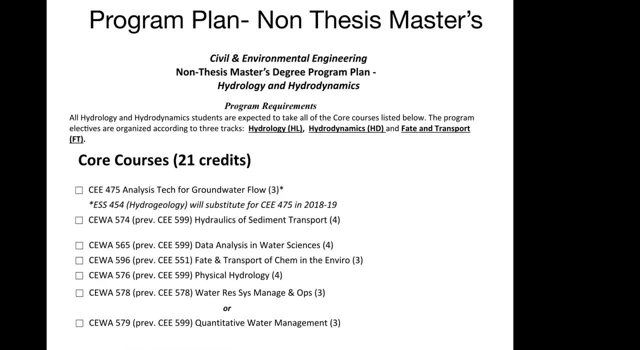 Data analysis in water science, Fate and transport, Physical hydrology And the water resources systems management and quantitative water management. I mean these are largely the hydrology courses, But I see some of the hydrodynamics students and fate and transport students come and take my physical hydrology course, for example. 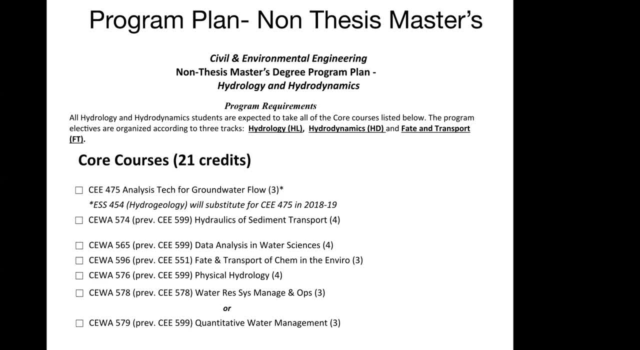 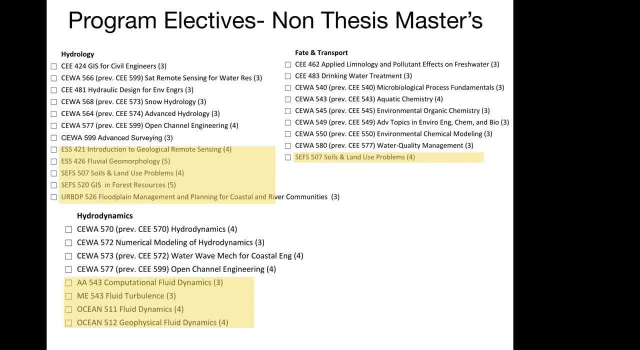 Or water management course. So the program is very flexible, But you have, like, the 20 credits that you talk to your advisors and we expect you to take, And a bigger list of that is that with respect to the three different tracks of these courses. 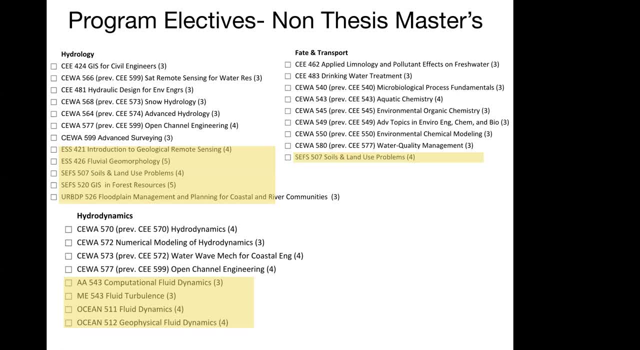 This is the list. Sorry, this is the elective lists. And these elective lists again. you, based on your interest, you talk to your program advisors And you can pick these elective courses in order to make up that 42 credit. And within that 42 credit, I think there's also seminar included in that too. 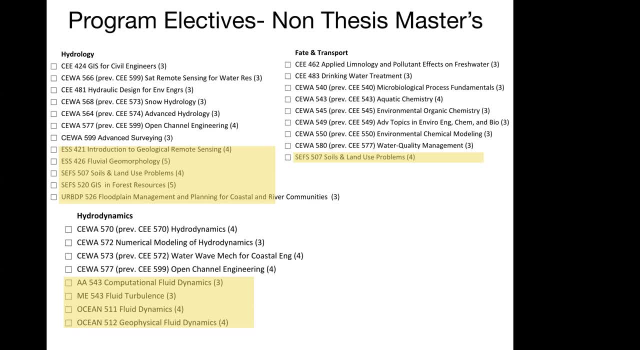 And 33 credits is the coursework essentially that you have to complete If you're doing a thesis. If you're doing a thesis, If you're not doing a thesis, then You just go up to 42.. You go up to 42 including one or two credits for seminar, right. 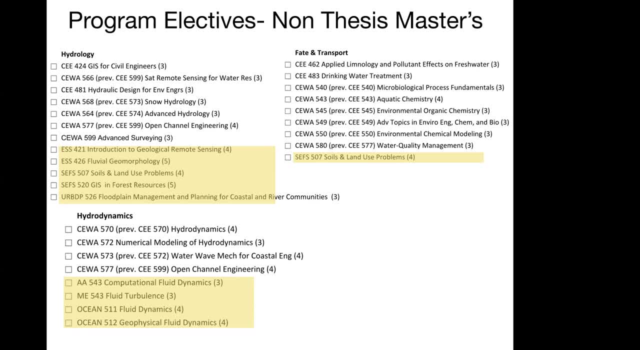 So in this list The yellow colored section is some of the electives that you can go and take from other departments. There are a number of electives from the earth and space sciences department, From the school of environmental and forestry And from urban planning. 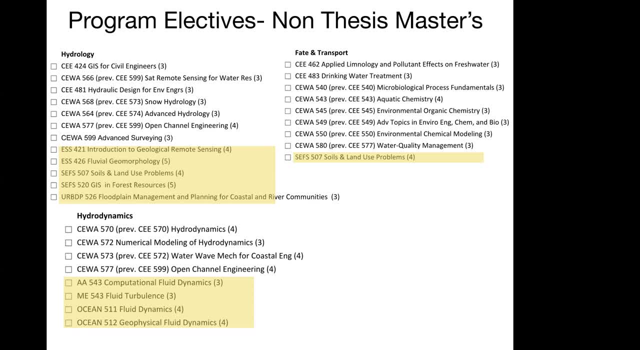 But talking to your program advisor and based on your career goals. I mean, if you come up with a course that you really want to take that's not in this list, That's totally fine. I mean, you can take. You can take courses from, let's say, from computer science department. 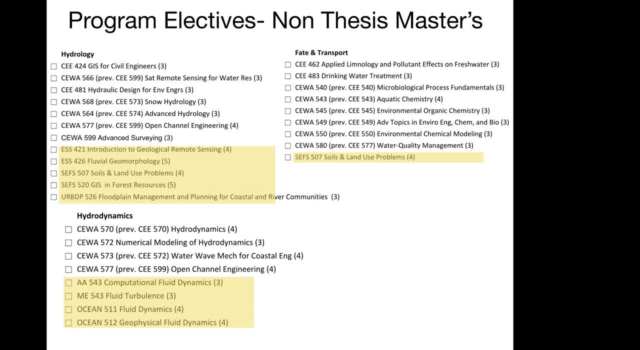 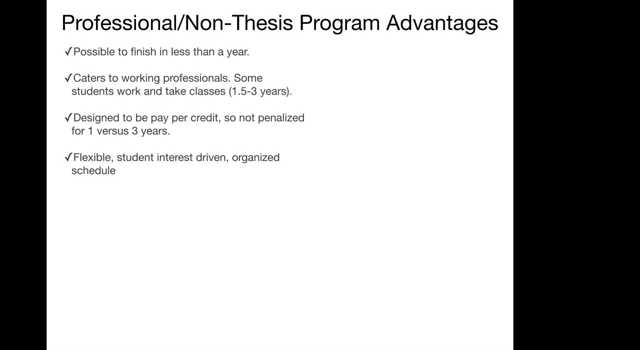 If you're interested in more data science issues or from the e-science. The advantages of professional non thesis program is that it's you can finish this in less than a year, Or within one academic year If you really want to do it in stance, and it's doable. 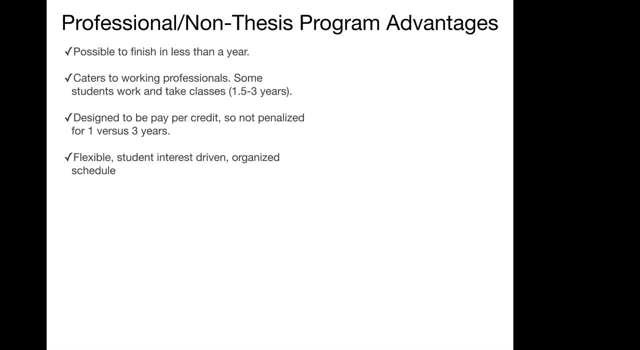 So we designed this program so that you can essentially pick it up, Yeah, And finish it within a year. But it caters to working professionals. Some students work and take classes, So you could do one course, for example, per quarter, or two courses per quarter. 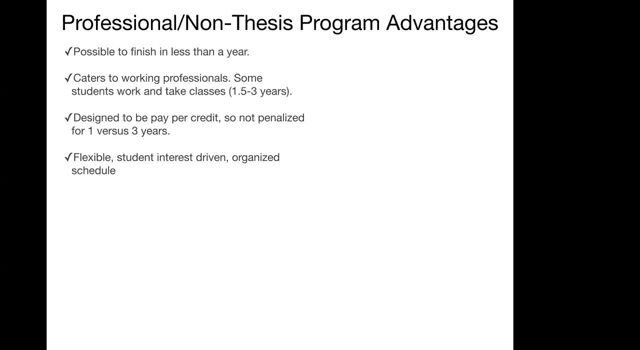 And you can do this for within a year and a half or more, Maybe within two or three years, depending on how you want to do it- And it's designed to be paid per credit, So you're not penalized if one versus three years. 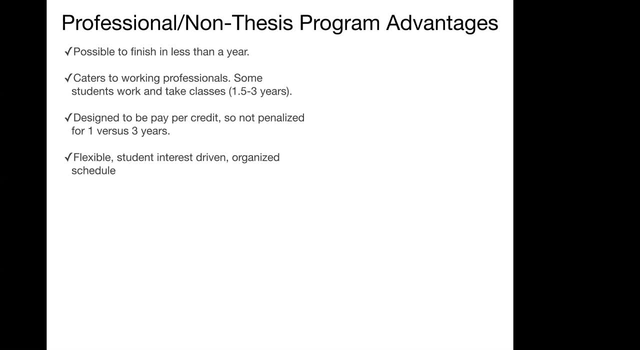 If you extend the timeframe to more than one, You just pay for the course And it's very flexible in terms of students. So the program is very flexible, like I said, based on your interest And your schedule. There are a lot of opportunities, both within the greater Seattle area in terms of work experience. 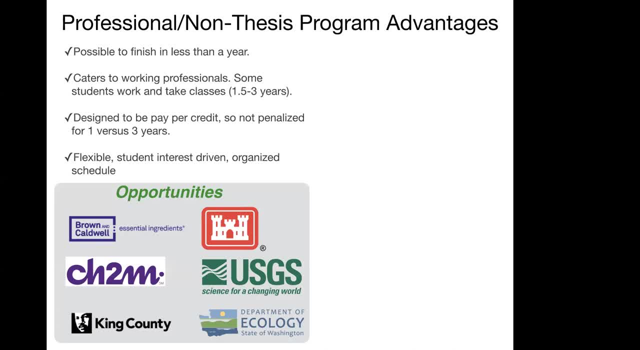 Within the Seattle area, Within the Washington state And elsewhere. of course There's a number of consulting companies, like Brown, and Caldwell is one CH2M. But, like Professor Brad also mentioned, There's a huge problem with the stormwater management in this region. 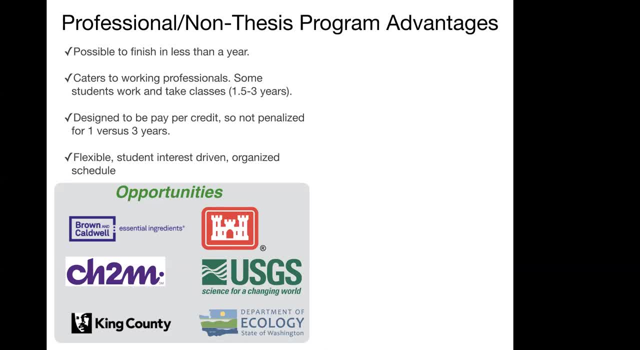 There's a lot of new project that requires new engineers and scientists, So there's plenty of jobs that are created in this region And there's opportunities with the Army Corps of Engineers, US Geological Survey, King County in Washington And the Department of Ecology. 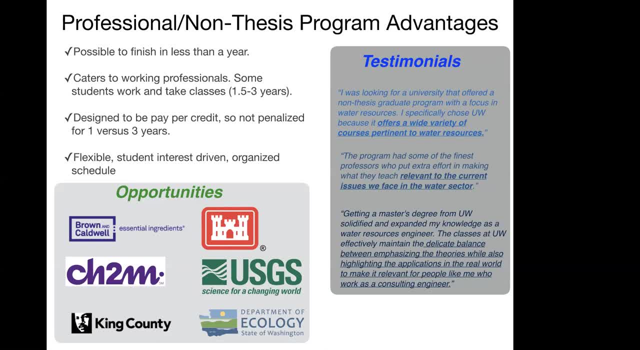 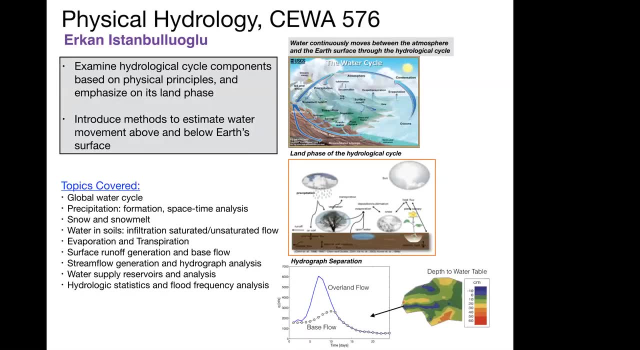 And there are some testimonials from previous years And some of the students that we encourage you to read before you make decisions. Okay, I'm just going to briefly go over the classes. Physical hydrology: That is the class that I teach. Essentially, it focuses on the physical properties of water. 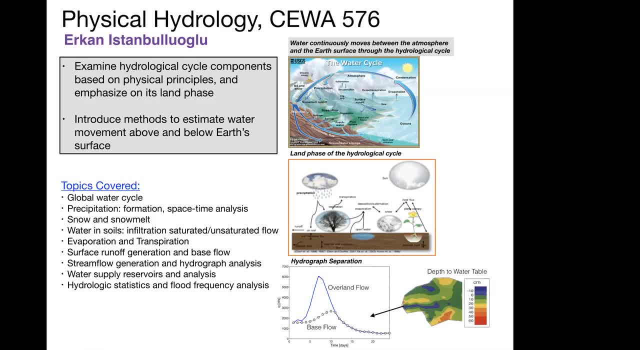 From precipitation to essentially the water gets to the water, lakes and lakes and oceans. We look at all the processes. It's theoretical based, Very fundamental, And I'm also integrating clotting And clot based computing in this class Because I have some project that relates to computing using browsers. 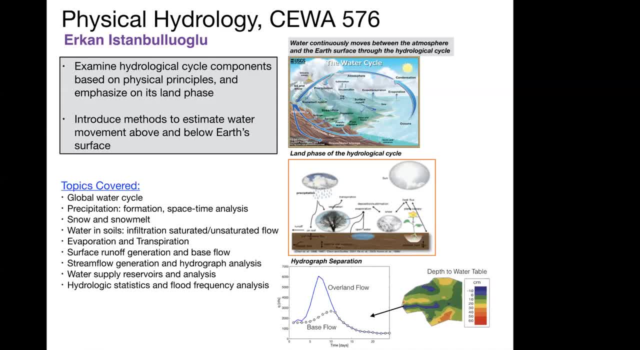 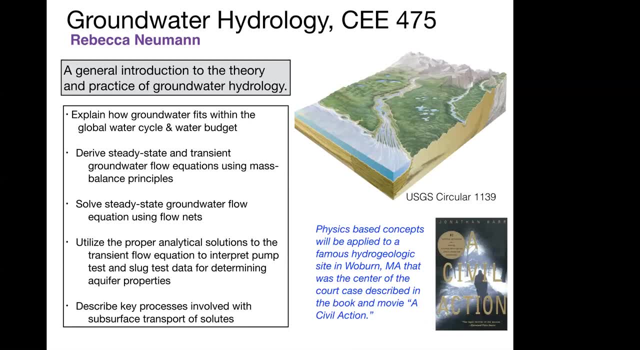 So we're looking at some numerical model applications Using code online. Groundwater hydrology- Professor Newman teaches this course. Again, look at the fundamental of groundwater transport And how contaminants also interact with groundwater transport. Open channel engineering is another fundamental course. 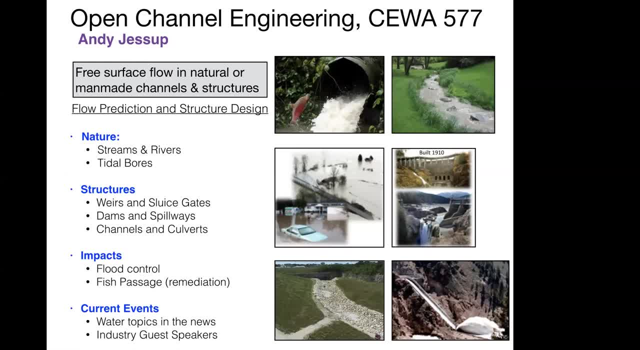 That we want our students to take. Professor Jessup is teaching And it looks at the natural streams, Structured or man-made streams in the built environment. It looks at the impacts of floods and flood control Studies, fish passages And they also look at more recent events. 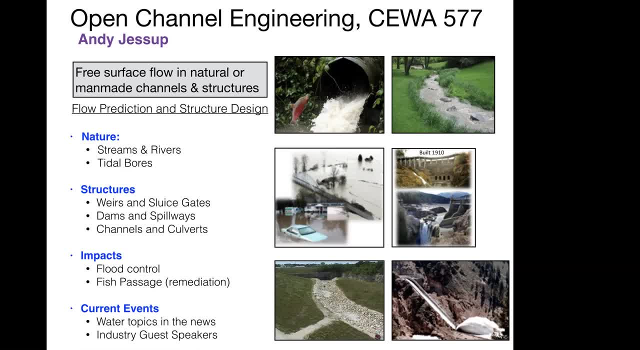 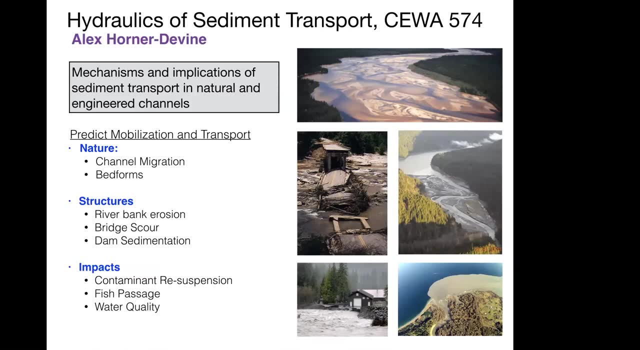 Like they have stories or anecdotes of the more recent events And they sort of build some calculation Analyzing more recent flooding events in this region. So it's very practical But also at the same time with strong theoretical basis. Hydraulics of sediment transport taught by Professor Horner Devine. 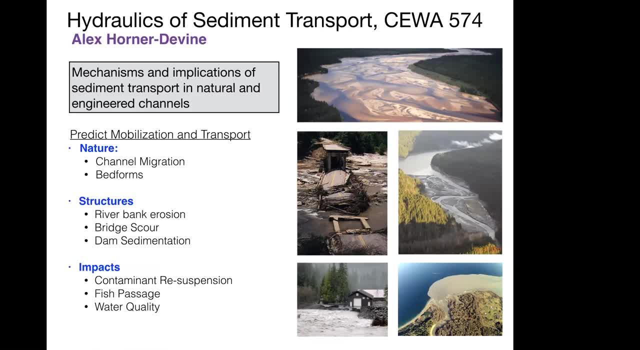 Again, both natural and the man-made systems are examined, But building on the open channel principle, Sediment is integrated in this. They look over different sediment transport And they look at the environmental conditions And their behavior in different systems And estuaries. 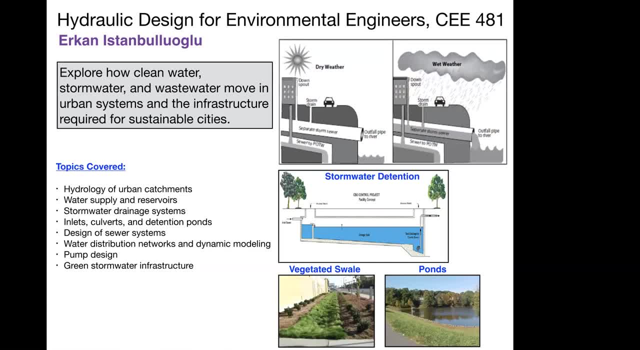 And where the streams meet the oceans. I teach hydraulic design for environmental engineers. I think this class is becoming more and more popular. In this class this is very practical solution oriented engineering course Largely And we look at the storm water systems. 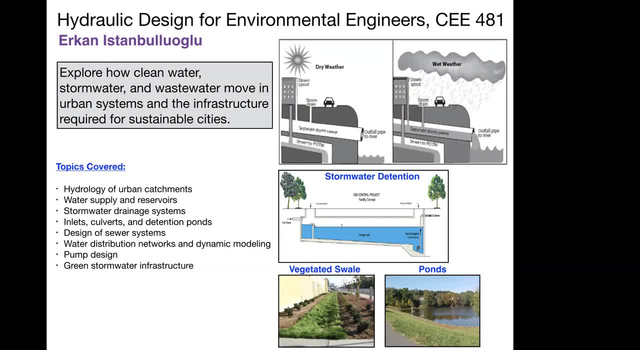 Water supply reservoirs, Storm water drainage systems. We look at pump design and green storm water infrastructure In this course. this is set up such that in every week we have a topic, Let's say pump design and pumping, We all go over that topic. 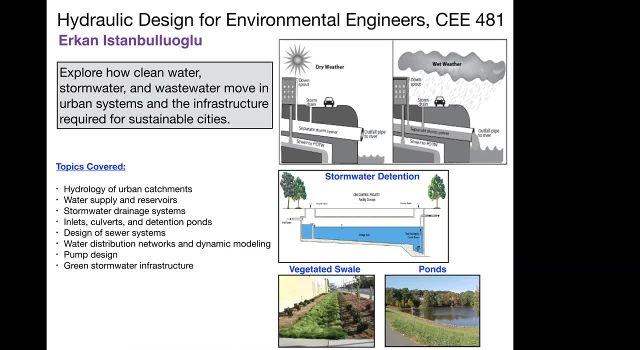 And in the end we have a software that we use. So we're looking at like roughly eight or ten software packages in this class And I talk to students, Graduate students, And they find this class very useful And they actually find it more useful than my physical hydraulic ones. 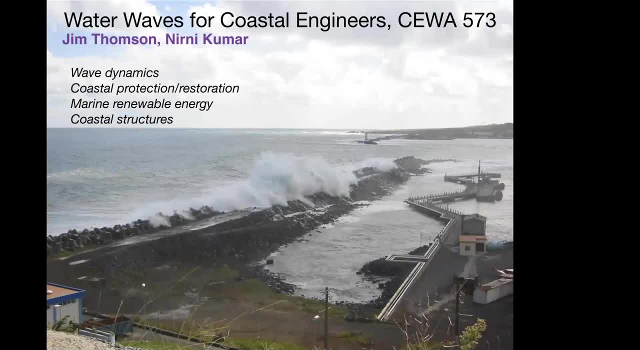 I didn't like that attitude, But I think that's fine Water waste. Water waste for coastal engineers Taught by Professor Thompson and Kumar- I think they taught it in every other year- And it looks at wave dynamics, Coastal protection and restoration. 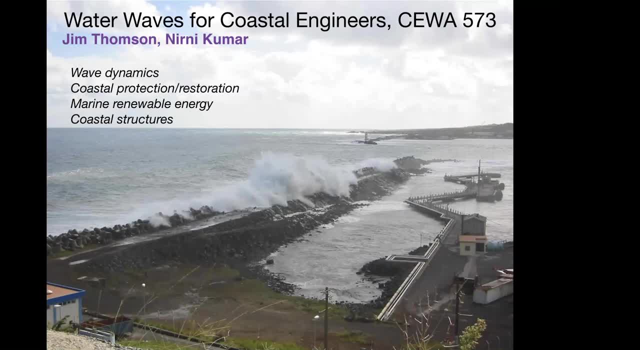 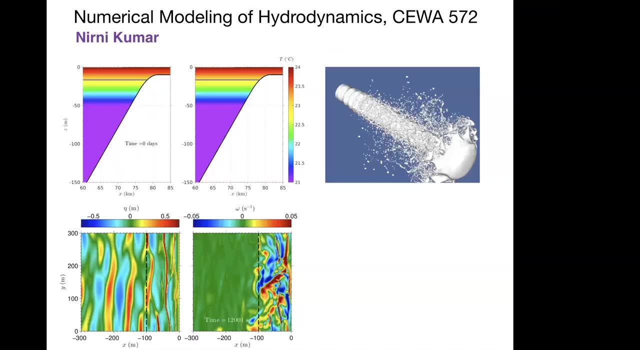 So it looks at the impact of waves in the coastal systems and coastal structures and the marine environment. Professor Kumar teaches a numerical modeling class on hydrodynamics. This one is fairly complicated. They solve partial differential equations for the movement of water Jets. 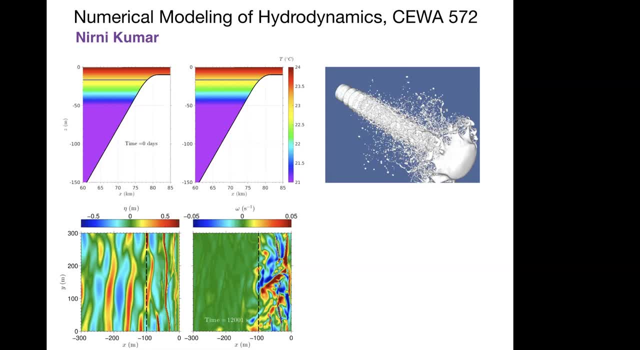 You know, the movement of sediment and so on In a very detailed, very fine resolution environment. that represents the domain integrated structure And they use like Navier-Stokes equations, Sandman equations and so on. So it's a very good course if you're interested in modeling. 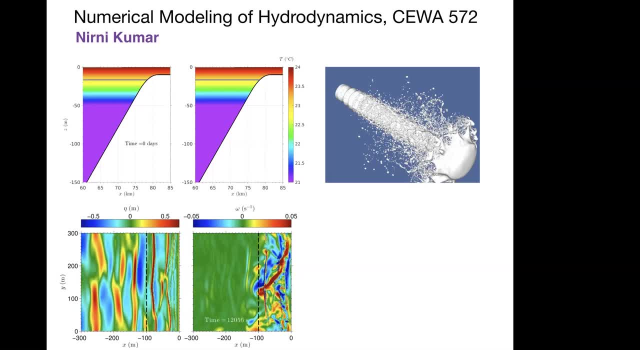 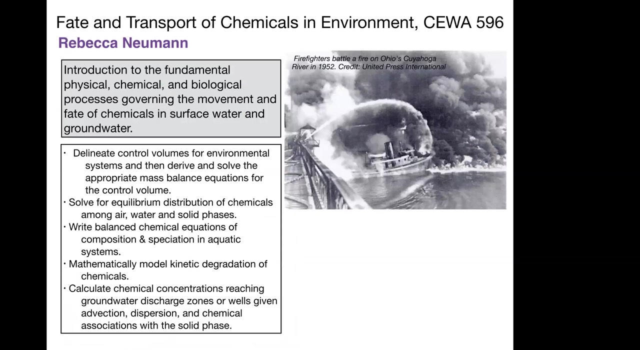 Here's some animation from a class project that was developed as part of this course, And it doesn't want to stop. Maybe it's because it's very interesting. right, We'll have to do a couple years here. Okay, There's also fate and transport, taught by Professor Newman. 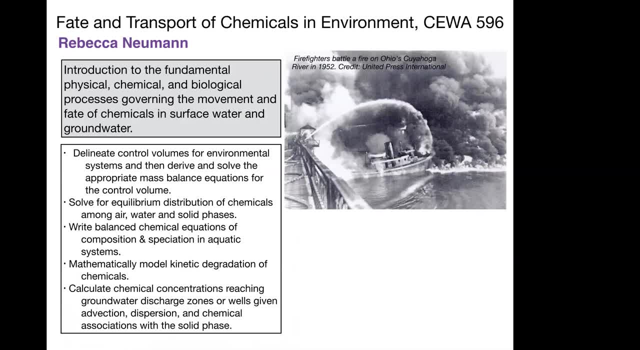 It looks at the concepts of contaminants and chemicals that's being transported And as the contaminants transport, some of them decay and others form and so on. But it's a very good introduction to the fundamental physics, chemical and biological processes that govern the movement and fate of chemicals in surface water and groundwater. 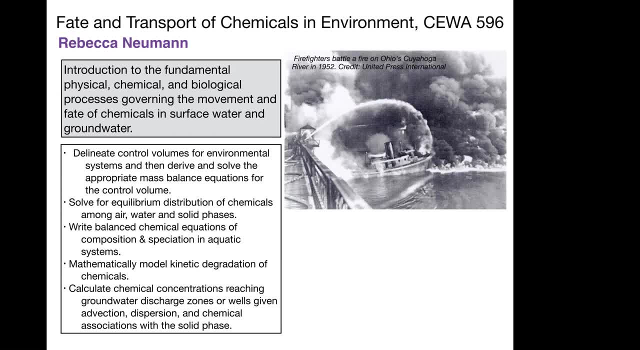 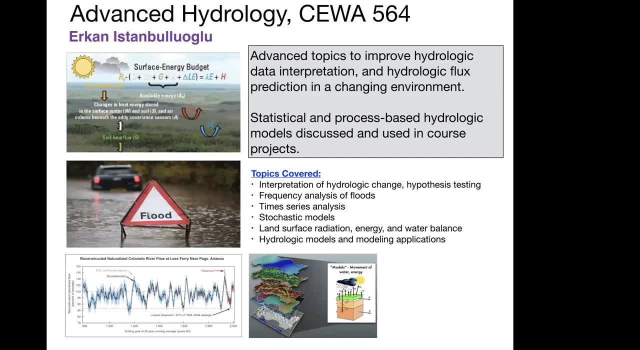 And she's got really great examples from the past events that involve transport of chemicals and outcomes in our environment- Advanced hydrology. I've been teaching this, but also in the more recent years, Professor Nice started teaching that too when I started alternating with some other class. 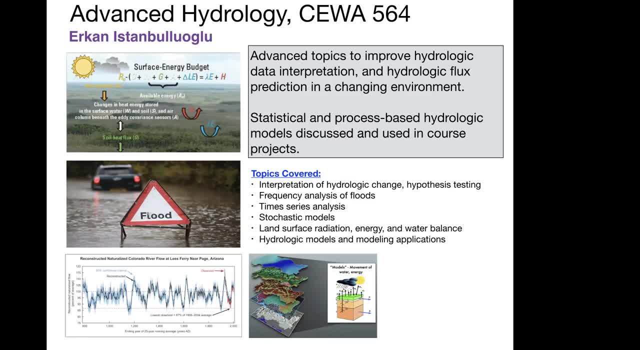 And in this course we have a very detailed description of the surface energy balance And we also have statistical models of the hydrological stream flow for the most part, And we also have statistical models of the hydrological stream flow for the most part. 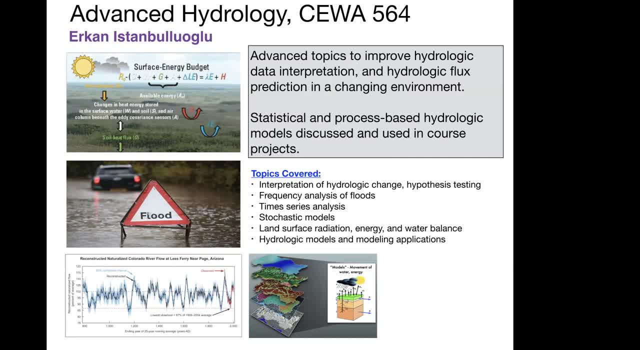 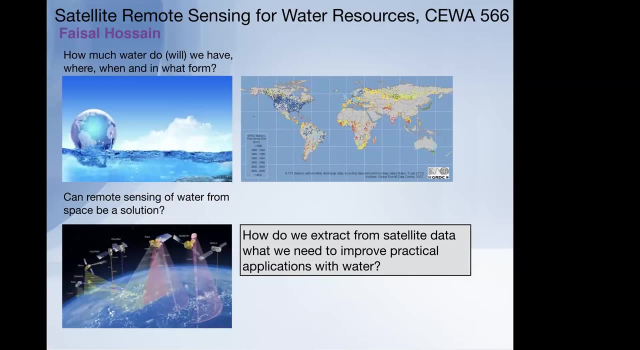 And we look into flood frequency analysis And we also have statistical models of the hydrological stream flow. for the most part, And this is largely a modeling course that looks at the processes- physical level processes- and the statistical processes- Satellite remote sensing, taught by Professor Hussain. 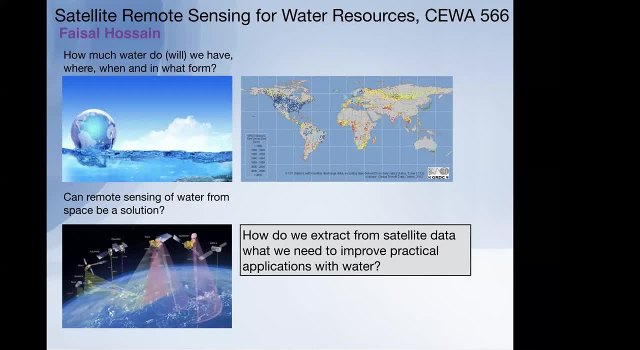 Their hands-on experience of using satellite satellite remote sensing data. I find this class very useful for my students who are doing modeling: a very good hands-on experience of collecting data and using the satellite data for hydrological calculations and estimating flood inundation and flood risk analysis. 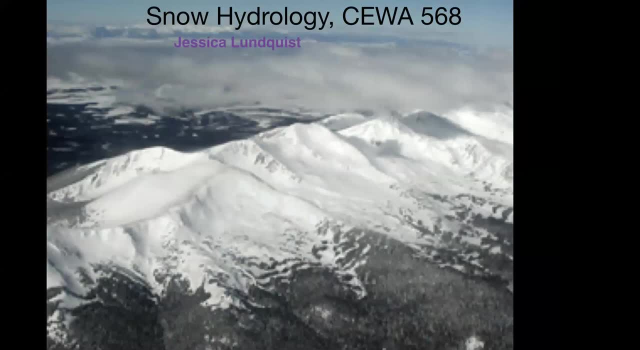 Professor Lundquist, like I said, she's an expert in snow and snow hydrology. She teaches snow hydrology course And in this course they look at the snow dynamics, including snow accumulation and sublimation processes and melt processes, distribution of snow in the fields through. 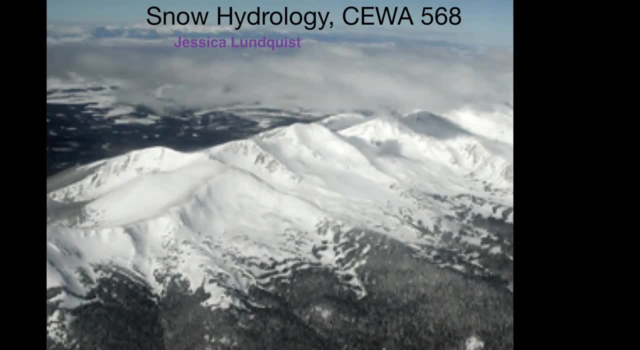 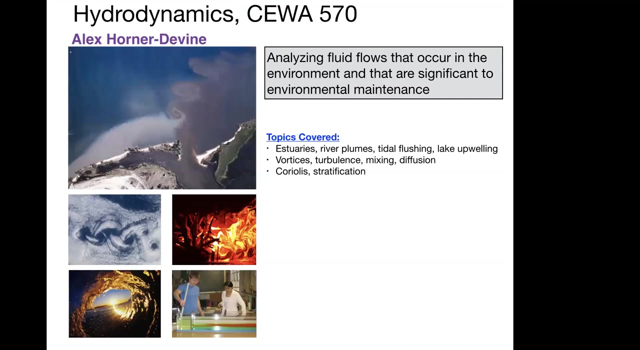 winds and topographic impacts and so on. It's a very critical course, especially for the Western US where we have large fractions of our water comes from snow from high alpine regions. Professor Horner-DeWine teaches hydrodynamics. 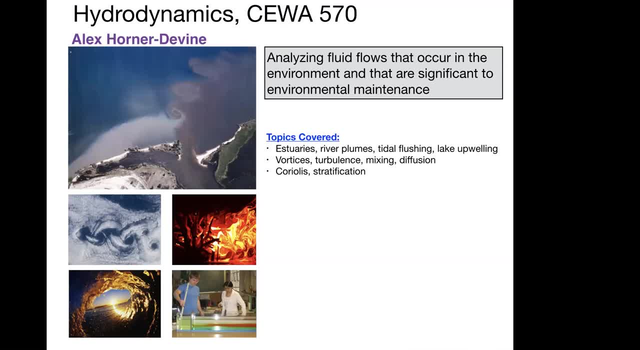 This course, like fundamental Theoretical theory, is about movement of plumes and sediments in rivers, in estuaries, river plumes, tidal flushing, lake upfilling and vortices and so on. You got a very fundamental view and a lot of data analysis in this one. 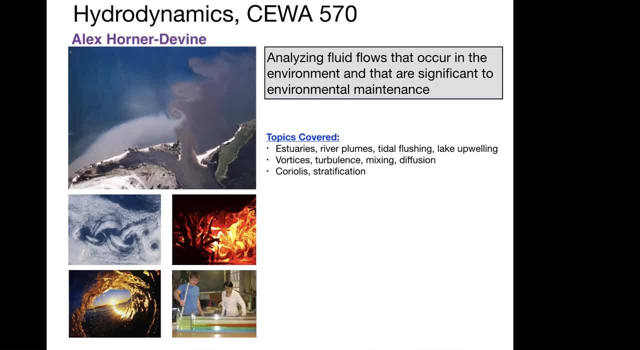 This doesn't have so much of a modeling context but heavy in theory and heavy in using actual observations to interpret measurements. So it's very important to have those measurements in relation to theory. Advanced surveying taught by one of our newer members, Professor Xun. 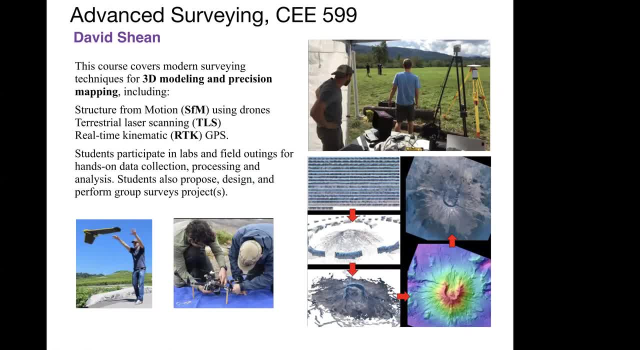 This class is a very interesting one Also. he teaches modern surveying techniques using structure for motion, terraserial laser scanning, real-time kinematic GPS's- And I'm also involved with the project with David, I mean, he has all these gadgets that he uses. 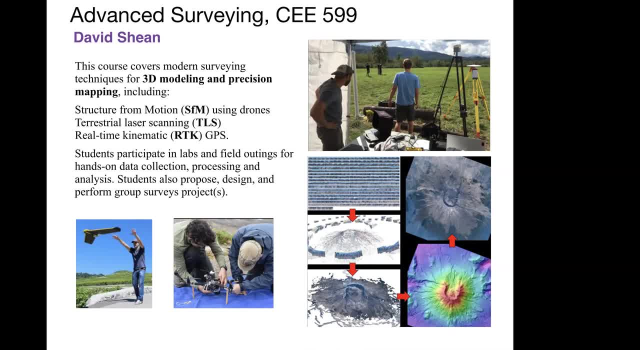 And I think it's important and I'm really glad that he's involved. I mean, he's involved with a lot of the science that he does And I think we're a very good team to create microtopographies on the landscape and changes on the landscape. 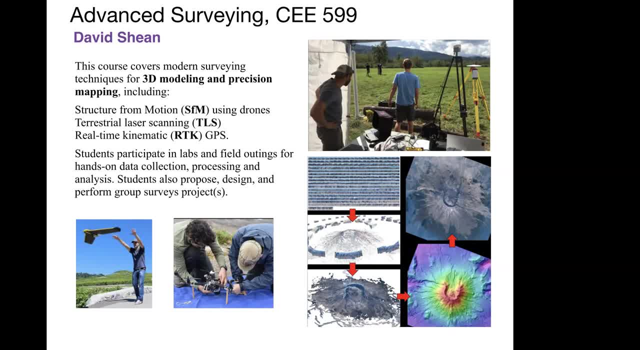 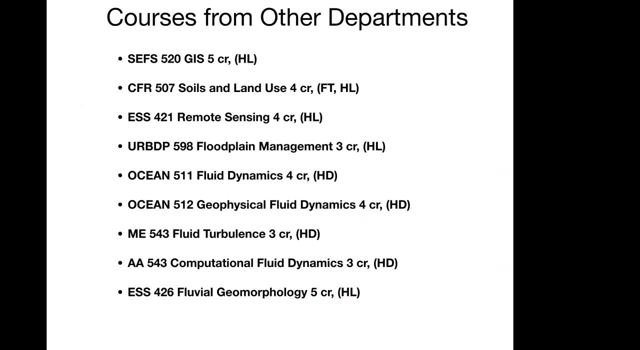 He also works with glaciers. He has a glacial time machine that he developed that he can track the evolution of glaciers, as well as the topography, through some of the methods that he develops and also teaches in this class. So this is one of the very interesting courses, modern courses, that we have. 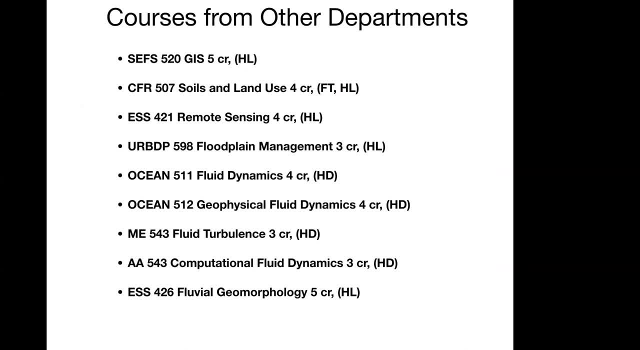 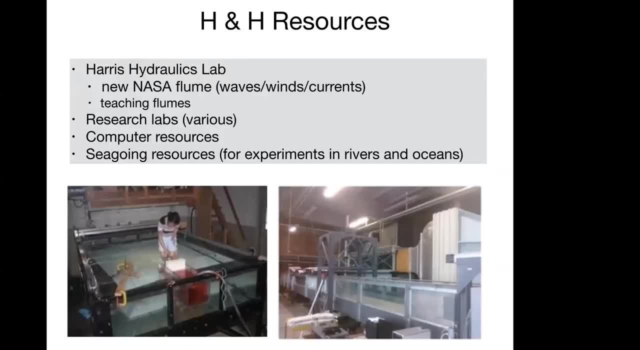 Like I said, there's a number of courses that you can take from other departments, that you can explore these in planning your program of study. In terms of resources, we have Harris Hydraulics Lab if you're interested in hydrodynamics. 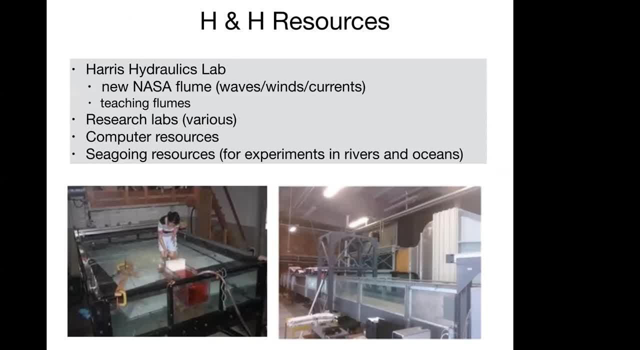 There's a new NASA flume that's right on the bottom right corner that can create waves and winds and currents. We also have a smaller teaching flume. There is the The flume on the bottom left that's more like a basin. 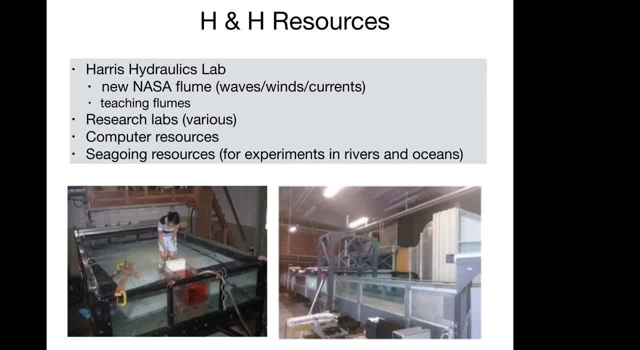 that is used for estuary experiments. We have plenty of computer sources in our department and across the campus And we also have seagoing resources in the Harris Hydraulics Labs, like the vessels to go out in the sea and the rivers to make measurements. 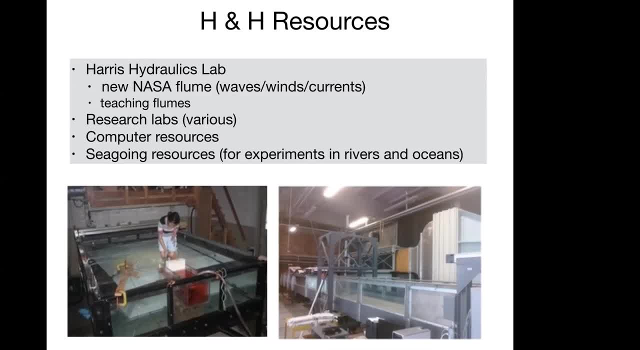 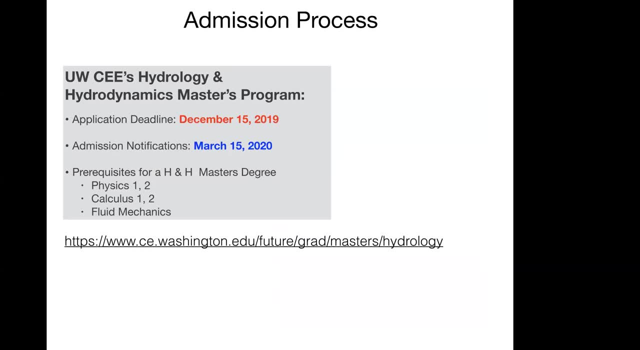 and ocean cruises and things like that for resource purposes. The application, The deadline: I'm sure Eric already covered some of these through other communications, but the deadline is 15 of December And the admission process usually takes like by mid-March. 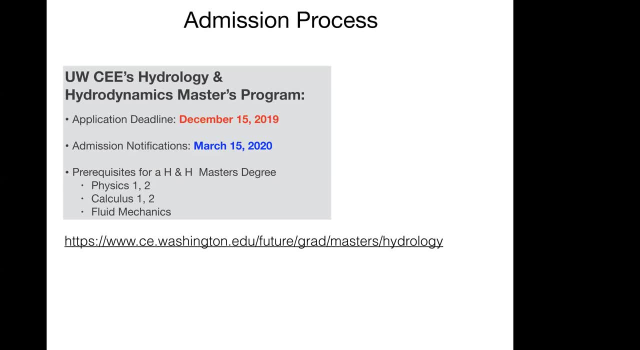 And for prerequisites for HNH master's program. we, like you, have taken physics one and two, calc one and two and fluid mechanics. We also teach fluid mechanics. So we've gone down fluid mechanics And we also teach thermodynamics one and two. 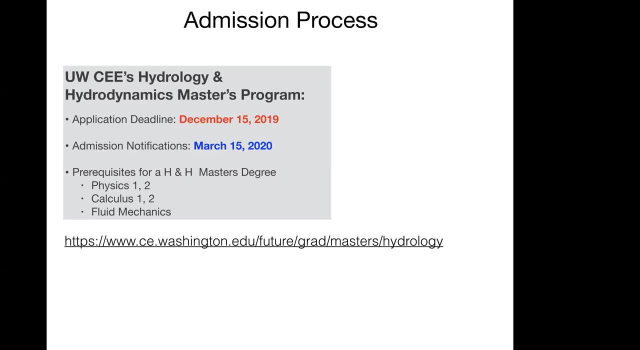 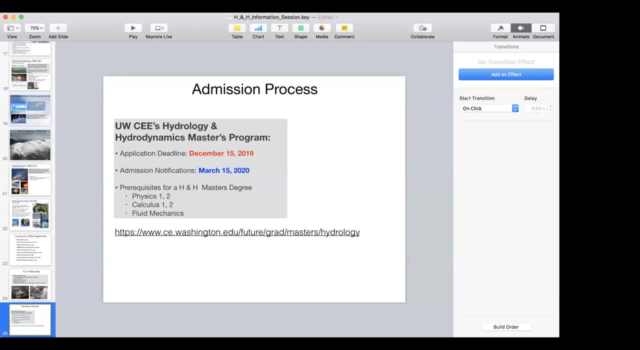 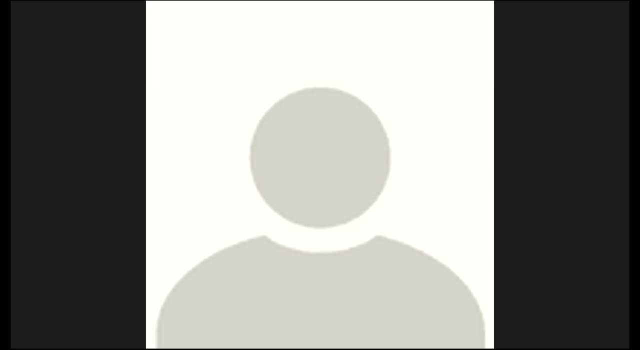 And then this is what I call the, And we're gonna bring in your students from Silicon Valley And we're gonna get some of your students from the University of Michigan And we're gonna get some of your students from the University of Michigan. And we're gonna get some of your students from the University of Washington, And so I'm happy to see you. You're welcome to stay and talk with them, And I'd like to keep in touch with you in the near future as well. 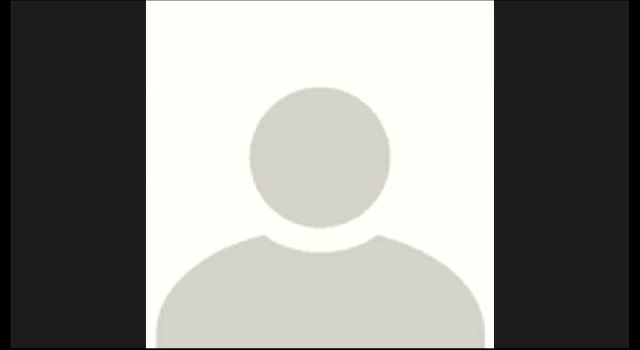 a class that has a focus on mass balance and also a class that focuses on fluids, and we offer both of those. in our department, we offer mass balance classes all three quarters. we offer fluids all three quarters as well, or at least two quarters. yeah, yeah. and so if you were to come into this, 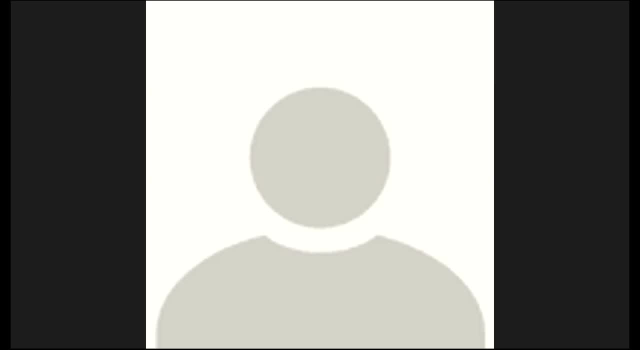 department from, uh, from a non-engineering background, we'd, we'd, we would um require that you take those two classes, just so that you get kind of on track with the kind of classic ways of of of approaching environmental problems. so from environmental engineering, i would say the 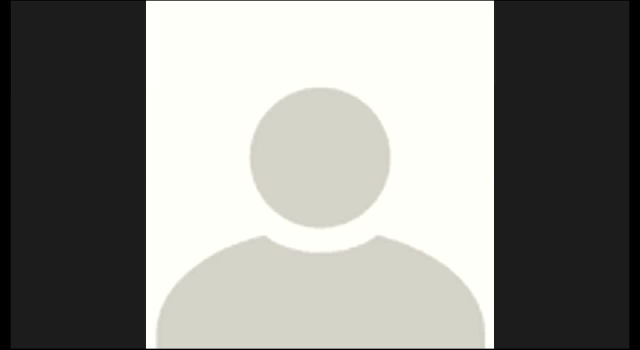 foundation of environmental engineering would be mass balance- mass and energy balance- and so you really need to learn that topic. so that would that would be our prereq. if you come from an outside field, great. so now, if you have questions, feel free to type them in the chat. um, we've taken them for a. 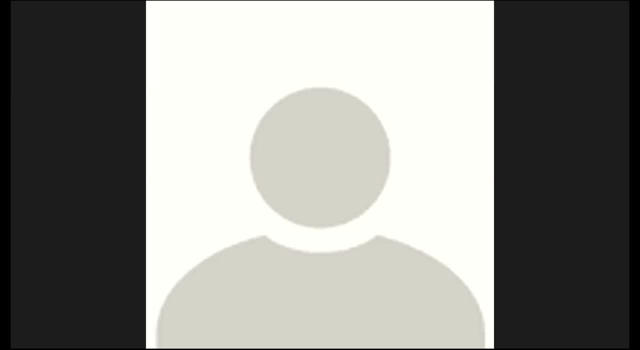 little bit. uh, to get us started, one question that's come up a lot this week you is: if a student is interested in a phd research track, do you recommend- and they don't have a master's degree already- should you think most students are best served applying for a master's? 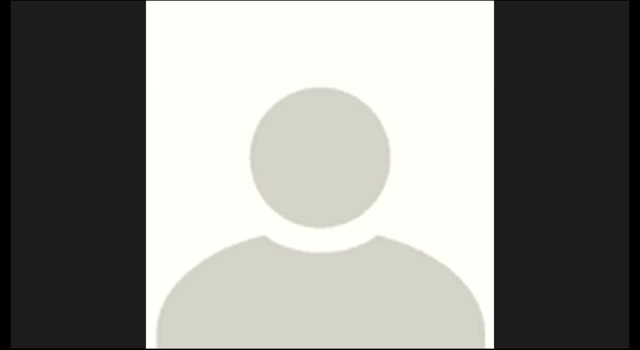 thesis uh option- and then stating that they have an intent to continue on to a phd here elsewhere, or do does your group, um, accept straight phd candidates? so, um, the the first point i would make about this question, about whether you'd try to pursue a phd track or or the master's track, is that there is. 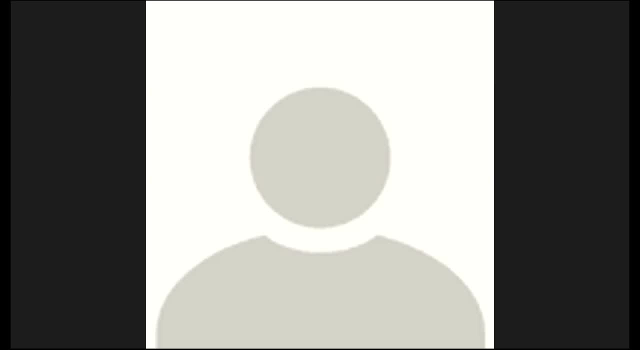 a lot more interest in our graduate program than there is funding available to support phd students. so not everybody that wants to come into our pro program could be supported on a funded project because there there aren't enough projects. but it's a very good idea to indicate your interest. 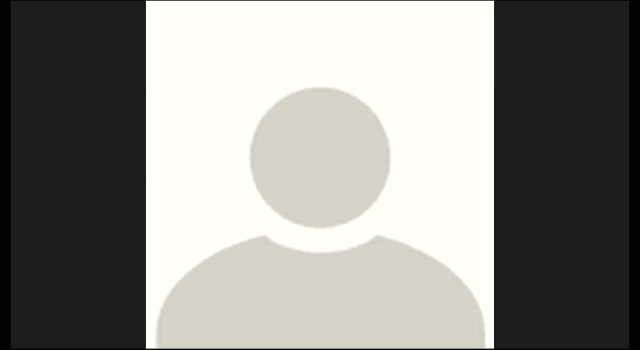 in ultimately doing um, a phd project. to be completely honest with you, i think the first thing i'd say is: um. the first thing is to give us a lot of insight into what you're doing, and you should be having conversations with us about what you're doing and what might be your look out for behind. 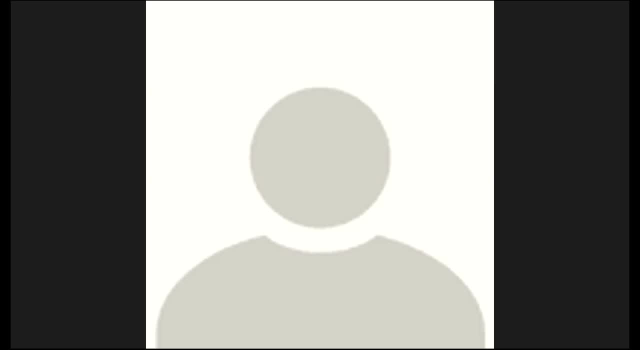 the scenes, as opposed to what you're doing in the future. um, again, i would say as much so you're doing, in case you need to go out and do a little research. uh, there's always a lot of what you're trying to do, um, and you're doing, and you're helping this group and then the race as well. 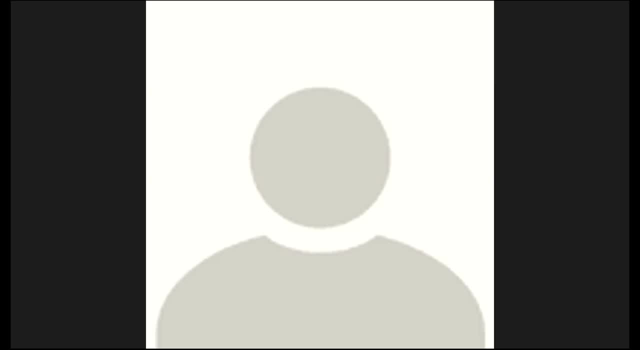 but you know we have a lot of interest in that and the reason- i think that's what makes uh phd students really interesting- is that you know we have a lot of students and they've been doing, you know, every other course they've been doing. but i think that's just one thing. that's really. 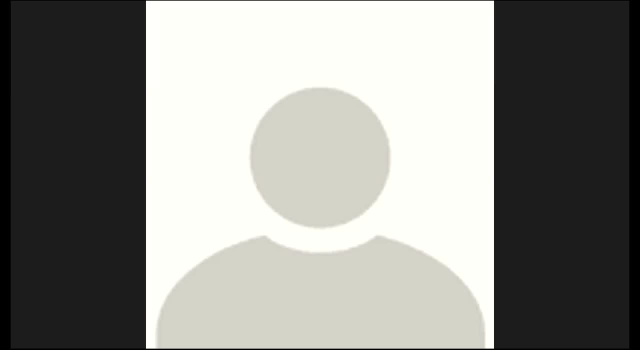 important for us today, um, in terms of you know other things that you're doing that you're able to do straight in the door. Another thing that does happen is a you know it's common for professors to recruit PhD students out of our current pool of professional master's students. If somebody has 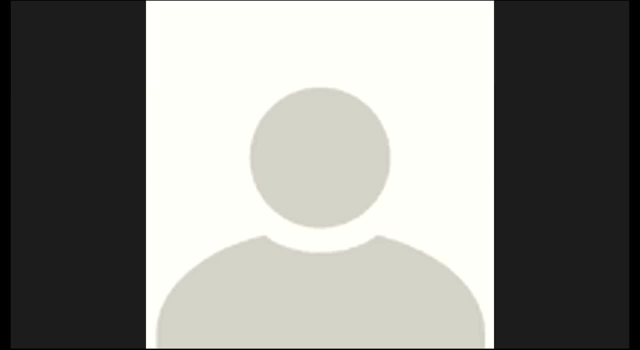 a student in their class. it really seems like they're enthusiastic about a topic that professor has funding for. then that might be the best fit for the project. And that happens a lot. I would say. I don't know, maybe half our students get recruited out of the professional master's program. 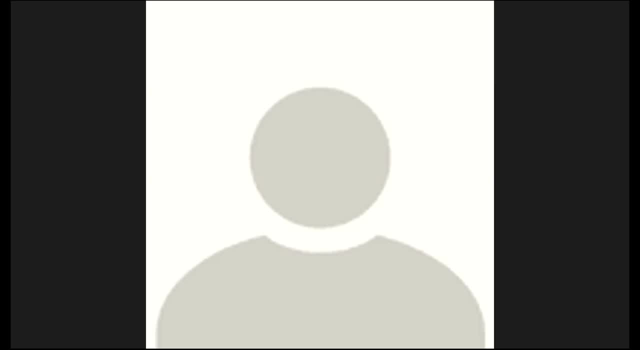 but not all of them. not all the professional master's students end up doing a funded research project, And you know a fair fraction of them don't want to, because they come here and they want to get out into the job market as quick as possible And the easiest way to do that is to 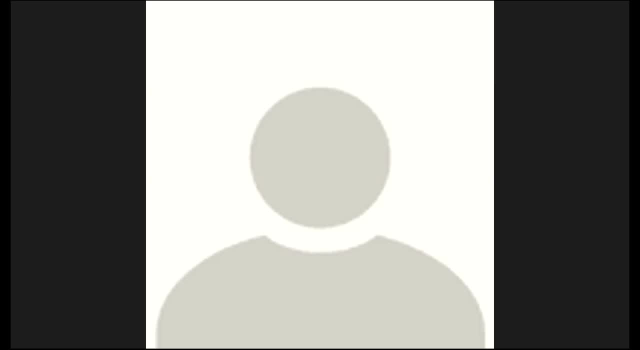 come in here and to finish up in three or four quarters or, you know, finish up in two years and work part-time is a very common scenario for the students that come in here. So both options are available. You know, if you ultimately do want to do a research project, then the best advice is really. 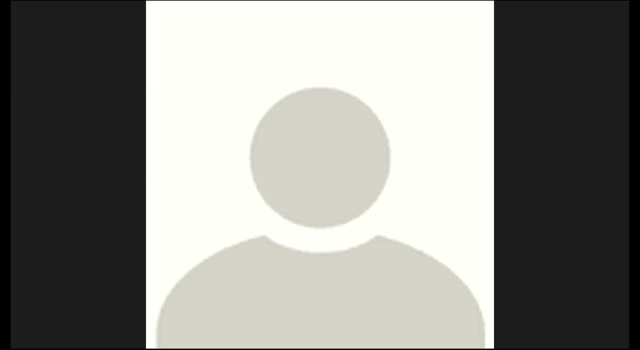 to get to know the professors and find out what kind of research they're doing and look for opportunities that really line up with you, know your interests and the project that's available. Those fellowships are available for PhD students- departmental fellowships. 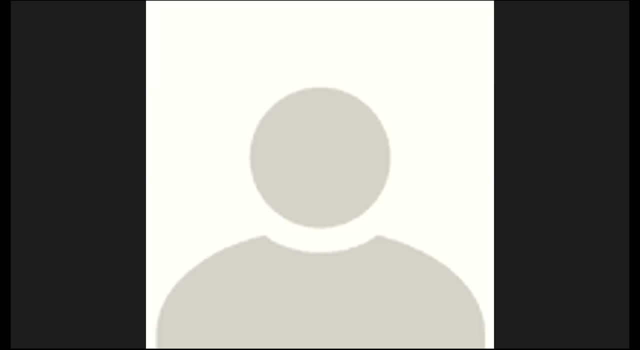 Yeah, there are also department fellowships to support graduate students. We have a question here. Yeah, I'm asking about GRE scores. I can speak to that. We do currently require the GRE. The test needs to be taken before December 15th, but the scores can come in a little after that. 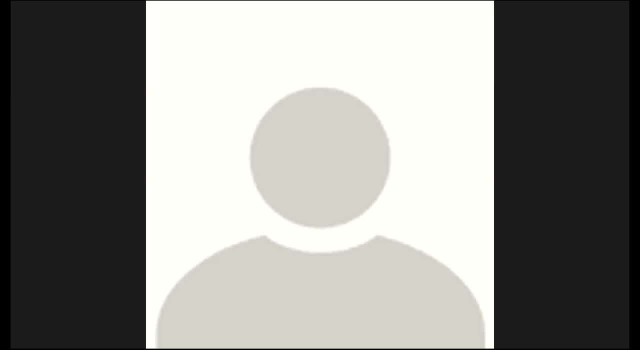 Usually it takes a little bit of time to process the application, So you should take the GRE about a week, at least a week before the deadline, but you have up until that point. I can answer the second question. So the question is: how can we learn about other groups in the CE? 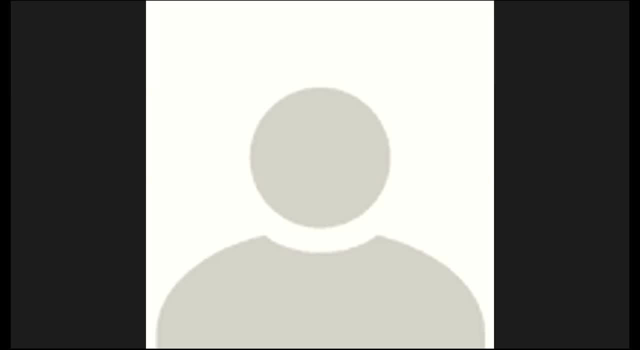 I'm the graduate program coordinator, so I'll talk about the various tracks that we offer in this department. We, you know civil engineering departments tend to be pretty diverse, And so we are offering master's degrees in a wide variety of fields. 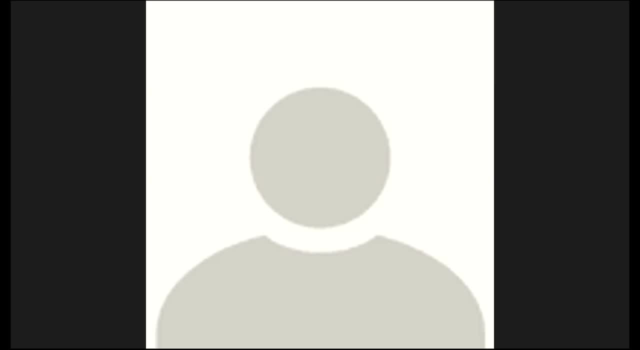 The largest group is structures. The second largest group is environmental, but we offer graduate degrees in structures, geotech, transportation, construction, environmental and hydrology. The environmental and hydrology groups overlap quite a bit, which is also the reason that Professor Istanbuli and I are speaking at the same time. 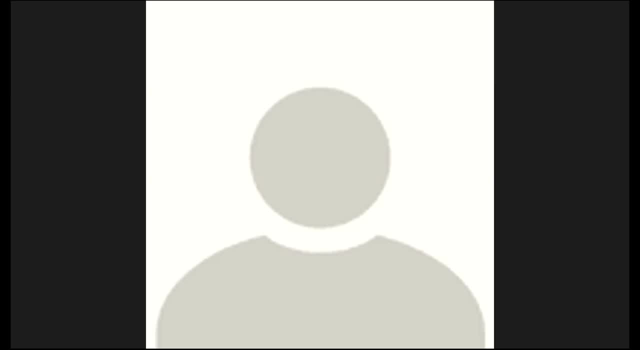 So students in those two groups often take classes across groups. There's not too many structure students that would take an environmental class. That's not going to happen too often. But you know we do have the six areas. Two of the areas are very closely aligned, I would say. 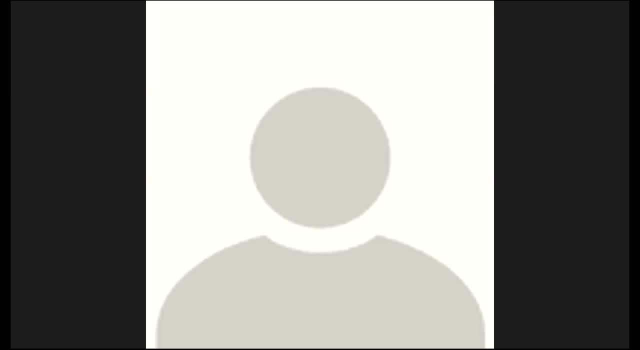 But if you go to the department website, you can find information for all Six areas And if you have any questions about that, that's something that Eric can help you out with as well. It's directing you to more additional information. Yeah, so this is also a good time to remind you that we have a general graduate advising email address. 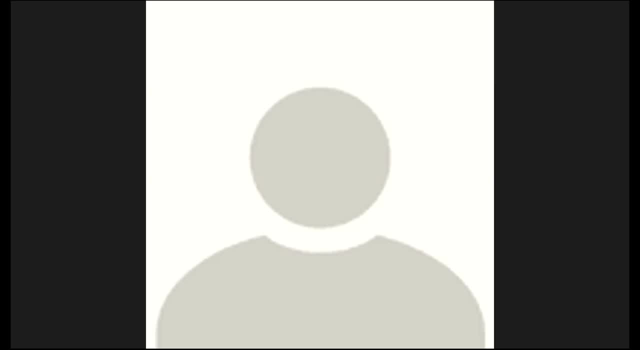 It's CEGINFO C-E-G-I-N-F-O at UWedu And that's monitored by me and the other graduate advisors. So if you have good questions- for you know process things, we can answer that. If you have good questions. 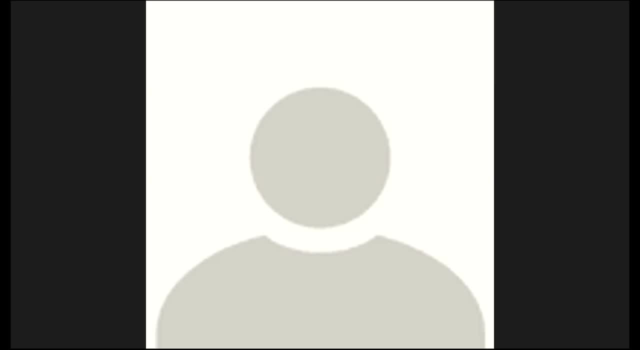 If you have questions for kind of more content areas, we're happy to forward that along. where we don't have the answers. Yeah, so there's. yeah, there's a question here about international students and TOEFL scores, which is English proficiency. 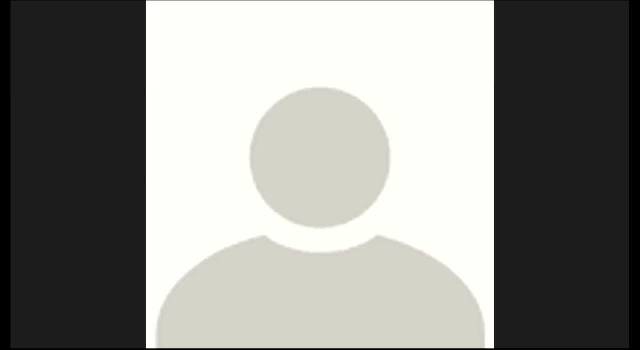 If you have a degree at the time that you would start the program. so, in this case, autumn 2020,, from a US university or a university where the proficiency, the language of instruction, was English, you don't need to take the TOEFL exam. 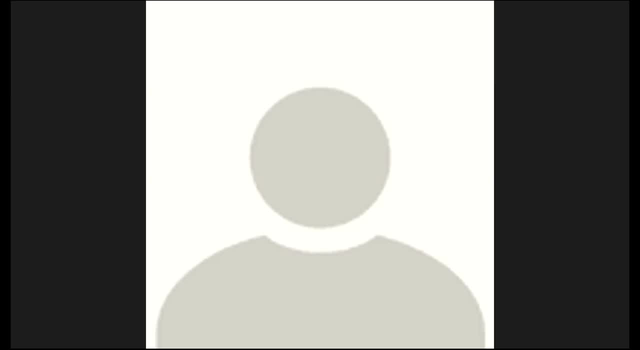 So as long as, by you know August, you have a degree, either bachelor's or master's, from one of those universities, you should be fine. I can answer this one. So this question is: are there students who have gone from non-engineering undergraduate programs to your PhD program? 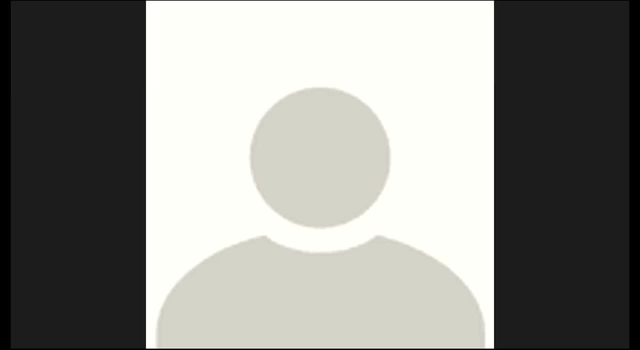 and have successfully attained engineering licensure after graduation. Yeah, many, Yeah. I would say most of the graduate students that come into our program from a non-engineering background are doing it because they want to ultimately end up with engineering accreditation, And so I would say most of them do that. Yeah, And once you've obtained a master's degree from this department, you're qualified to take all the engineering exams. You know you can take your fundamentals of engineering exam while you're still a graduate student. And then you know your PE requires a professional engineer's license. 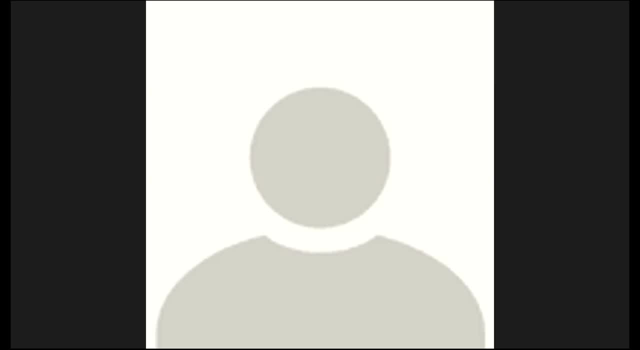 It requires some years of experience, but that's absolutely possible And I think that's the main reason many students come into this program from a non-engineering background is that they want to get that engineering licensure. licensing Okay, Incoming students without okay. 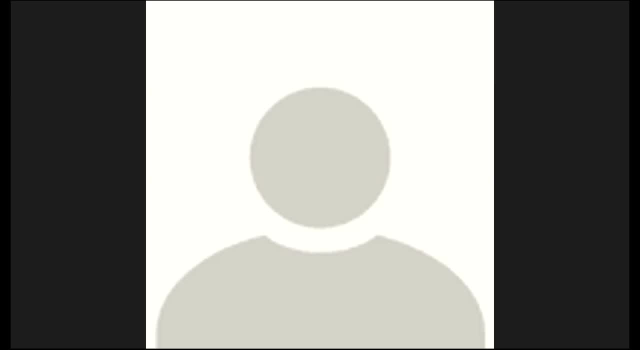 For incoming students without an engineering background, would the two prerequisite courses need to be taken first quarter of the program before commencing the core classes In hydrology? Is that like the fluid mechanics? Yeah, Yeah, I think. so I think we would encourage you to take them fairly early on. 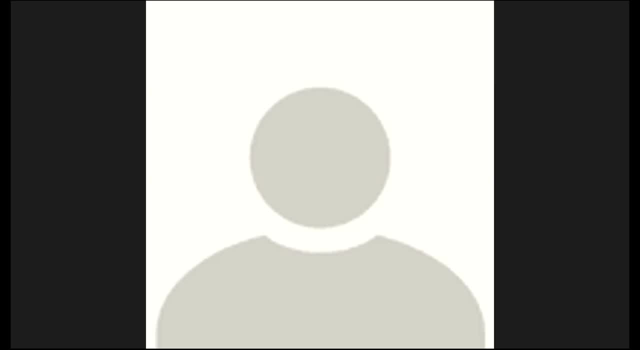 So the first quarter would be ideal, but you could probably take some of the hydrology classes at the same time. I believe, Yeah, you can take it at the same time, Or you can. I think there's a way that you can also audit that course, because that's a 300 level course. 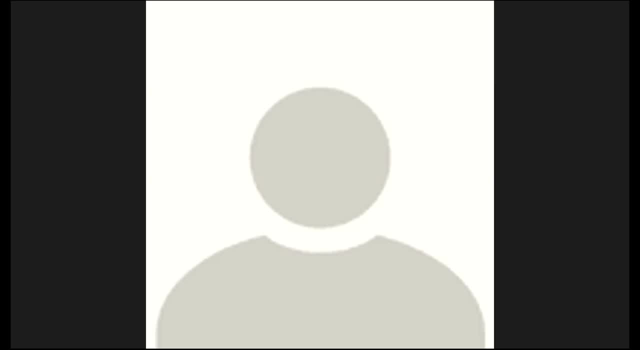 We just want to make sure that you have some background in fluids and hydrology And in hydrology and in open channel and hydraulics of sediment transport. we do have. we actually teach hydrology hydraulics, But in fluid mechanics you have a sort of a more fundamental background. 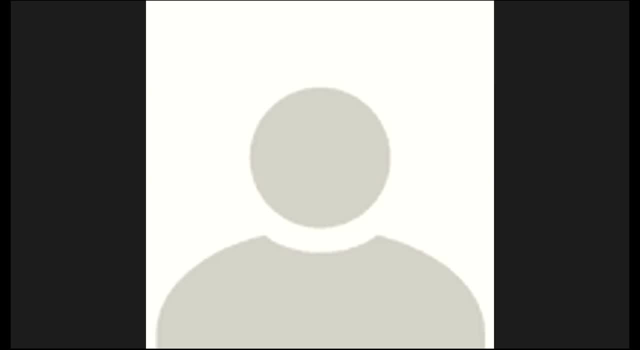 So some students do audit that course, Some students take it in combination with other courses, But there's a way that we can work around that, I guess. Yeah, so we encourage that you essentially come and talk to us if you have a situation like that. 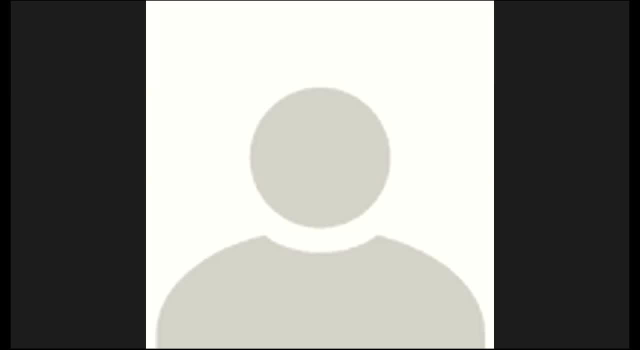 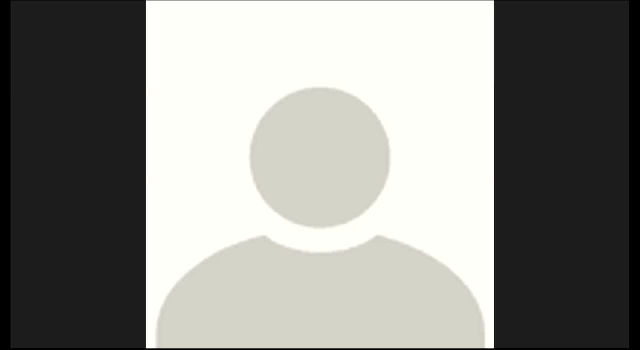 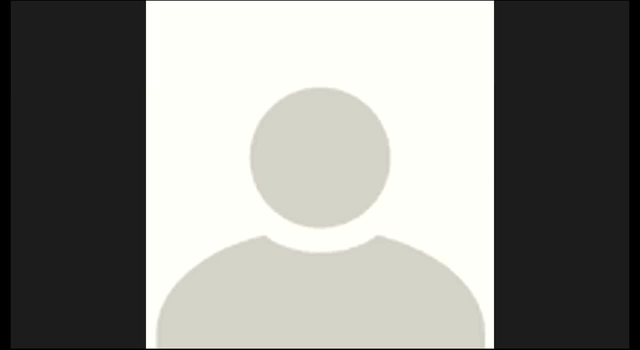 Degree. So what usually happens is students that are doing a PhD- I mean sometimes the students who are doing a PhD- will do a research master's as well, but it's also common that what they'll do is when they get 42 credits. 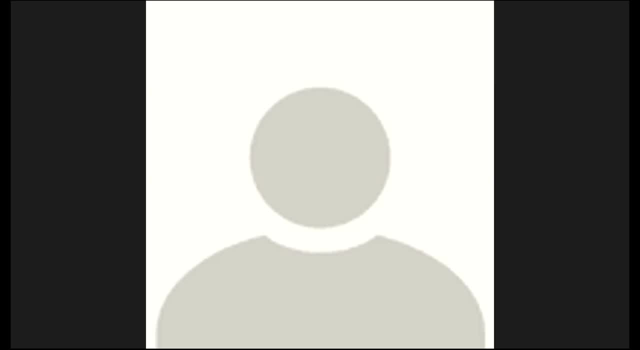 into their coursework. they'll get the coursework master's and then they'll just continue on and do the research PhD. So most students don't completely skip the master's. but if you want to, you could. It would just be a matter actually of not filing the paperwork to get the master's. Some departments on this campus skip the master's and go straight to the PhD, but I would say 90% of the students in the PhD also get a master's And it's always to the benefit of the student just to have an extra degree. 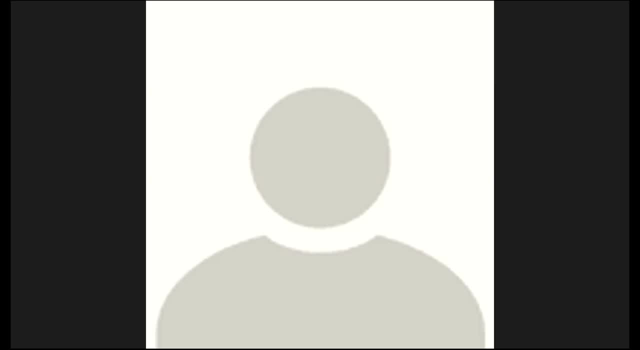 Yeah, So there's no extra time or cost associated with getting a master's along the way towards a PhD. No, it's just the paperwork that you need to fill out, And if you're interested in a master's thesis, perhaps- I mean- you may be working on a project- 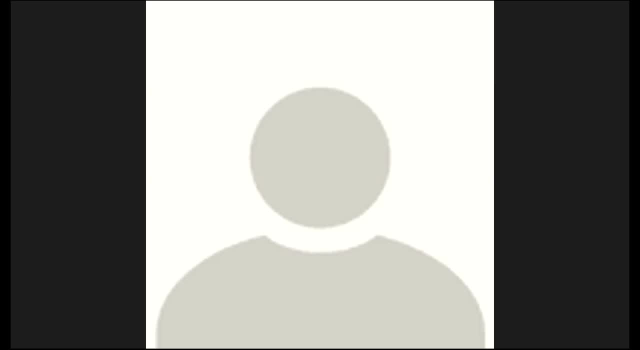 and you have your first paper and that could become your master's thesis paper. You publish the paper and have a thesis on that same paper, And then you perhaps move on to a different project or continue on the same project and develop three more papers or two more papers, and then you get a PhD out of those papers. 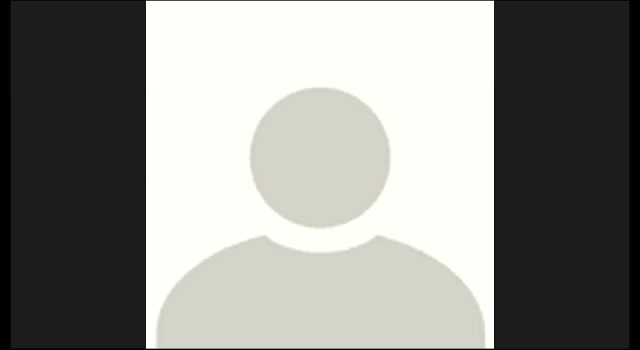 I mean, our program is very flexible and, essentially, as long as you can come here and be excited about the program and work hard and want to write papers, we'll have you. We'll find some other funding. Yeah, Any other questions? Any other questions out there? 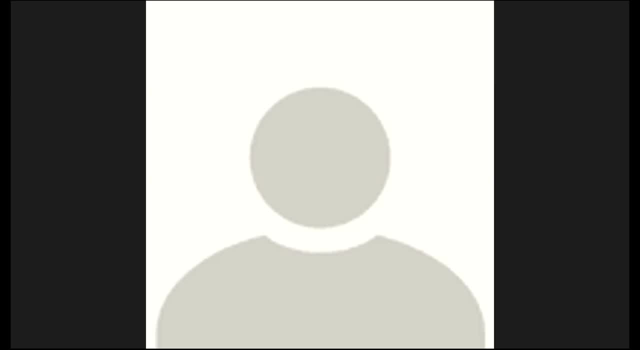 Any last words of wisdom from the two of you? I think also there's the data science option. Oh yeah, The programs too. Yeah, So there's a new thing going on, And do either of you want to talk about it? I'm happy to talk about it too. 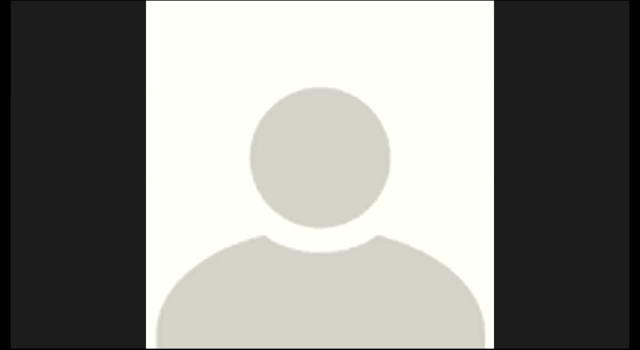 In our hydrology and hydrodynamics program. I talked about Professor Sheen. He's an expert in application of data, of big data sets in terms of representation of the geospatial variables, So he pioneered a data science option, And how it works is that we have some departments, of course, that can come towards the data science. 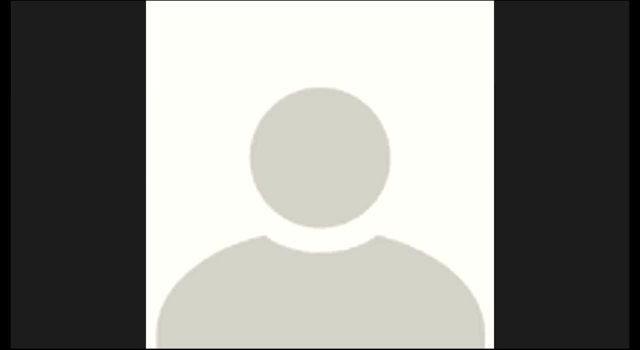 option And you take, I think, three or four credits of data science courses And two of them could actually come from this department, from the courses that you will already be taking. as far as the courses, One will be Professor Sheen. 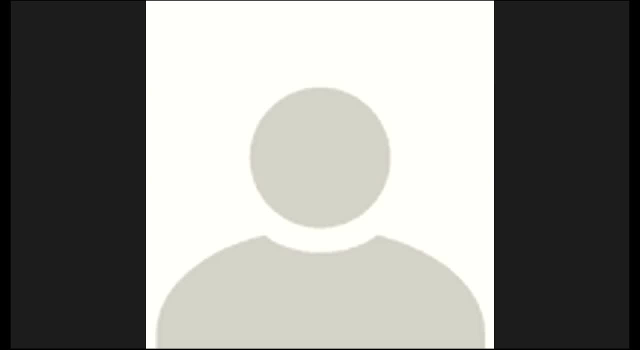 One will be Professor Sheen, Yeah, And the other one will be Professor Lundquist's course on data, on data science. And then you take two other courses from eScience And eScience. computer science professors offer those courses through eScience. 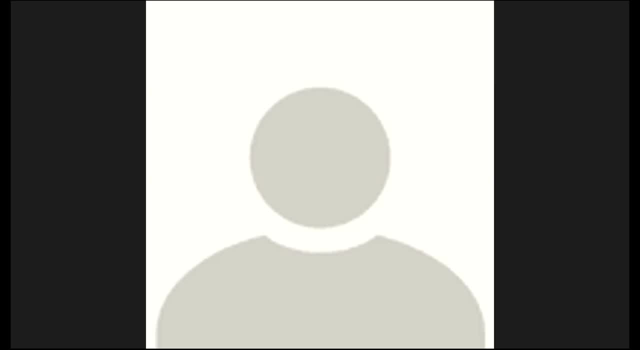 It may not be as difficult, as hard as a computer science student, but it's sort of a version that is more applicable for engineering scientists, more than just data, So I think that would be an exciting option, just starting in the next year. I can answer the next question from Rico. 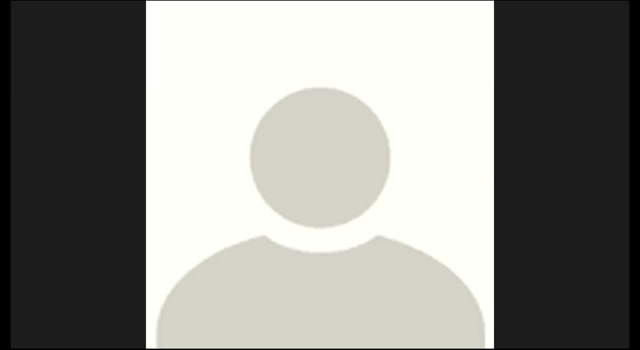 Rico asks or states: I'm really interested in water quality, water reuse and recycling projects. Which professor will be the best to be in contact with? Yeah, The people that would do that kind of stuff would be Professor Jessica Ray. Professor. 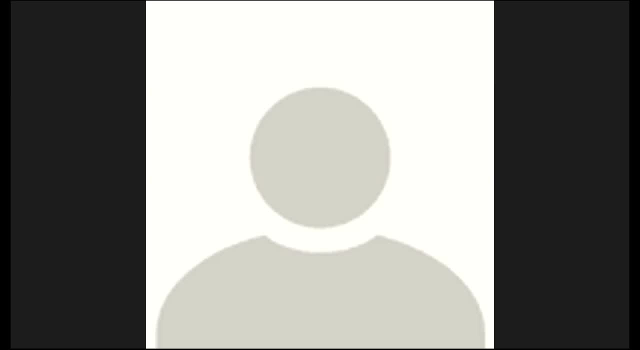 Mike Dodd, Gregory Korshen. I'm a water quality person, but more for natural systems. I'd also recommend that you look at Professor Rebecca Newman's profile carefully. She does water quality more in groundwater systems, But for the more engineered systems I would look at Professor Korshen. 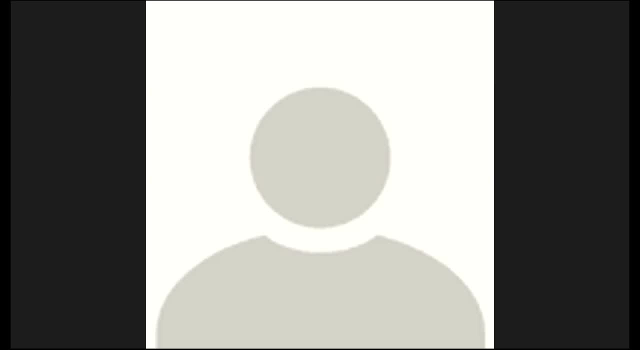 Okay, DoD and Ray, And also Ed Kolodji, has some interesting stuff that would fit in very nicely with this as well. Well, it looks like we are about to wrap up, So if you have more questions again, don't hesitate to reach out to ceginfo at uwedu. 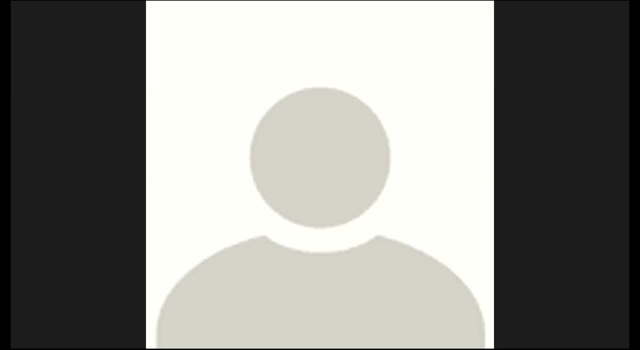 Oh, we got one more question. Did you ask that one? Oh really, geomechanics. Yeah, so we do have about five or six geotech professors, And so I strongly encourage you to look at what they're doing, And those are professors Joe Wartman, Steve Kramer. 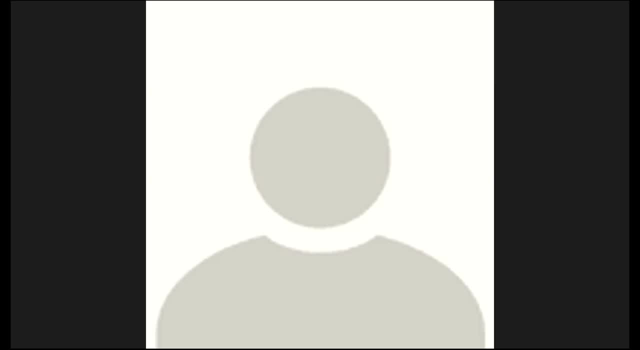 Pedro Arduino, Mike Gomez and Brett Maurer. So there are geotech And I would definitely look they're definitely doing some geomechanics. I wouldn't say any of us in the hydrology and hydrodynamics group or the environmental group are exactly doing geomechanics, Professor.